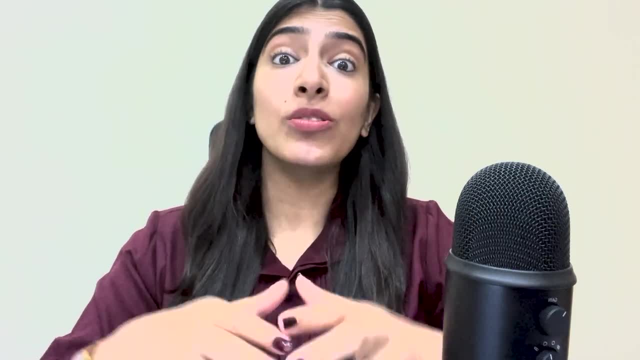 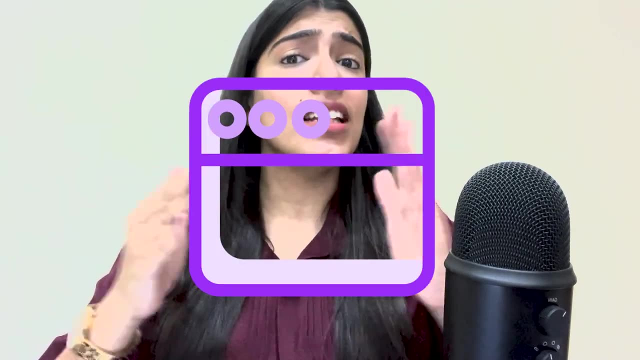 the name suggests we are going to be building things, But let's start with. why do we need build a design pattern and when do we need So? whenever we are building a very complex object which has a lot of configurations in it, we use build a design pattern Just. 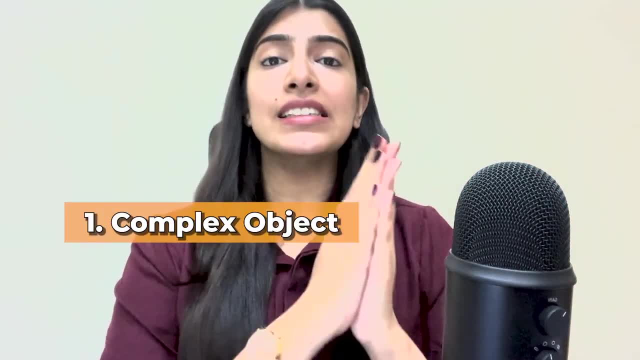 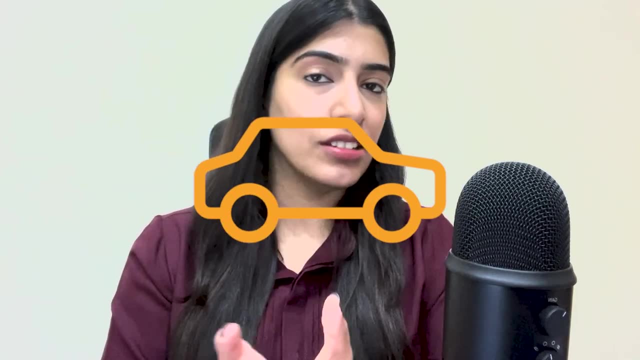 remember these two very important points. One is complex object. second is configurations. Let me give you a lot of examples. For example, you are building a vehicle Now. a vehicle can be a car, it can be a two-wheeler or a scooter, right, So all the vehicles have a. 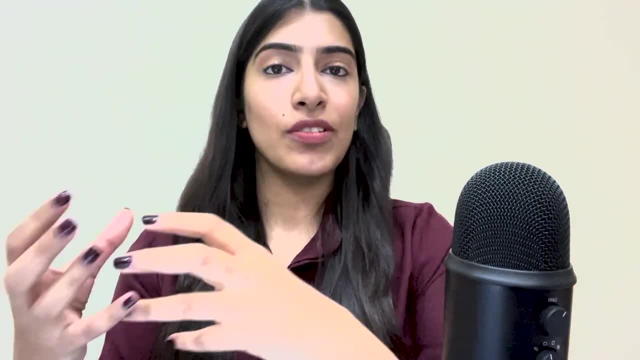 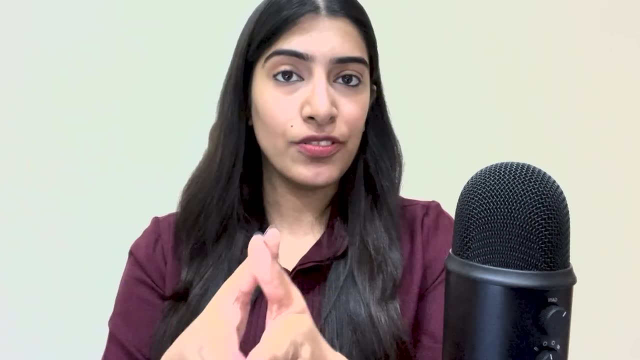 lot of parts to it. right, It's a complex object. For example, there will be an engine, there will be brakes, but the kind of engine that you will use for a car, and even within cars, for different companies of cars, and the type of engine that you will use for scooter. 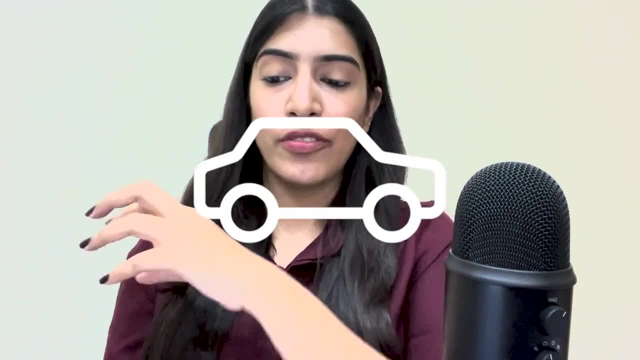 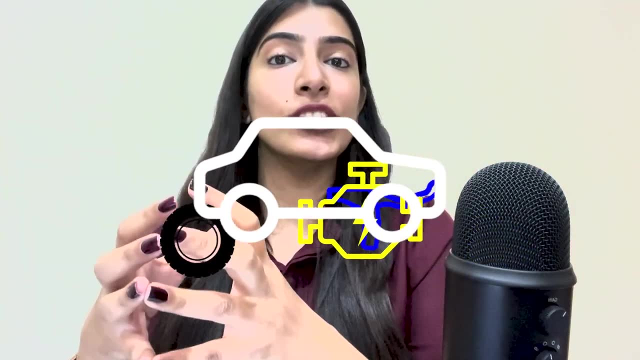 will be completely different, right? So to build a vehicle, you have to build parts of it, Like you have to build the tires, the engine, the brakes, all of that, and then bring all of those together to create the complex object, right? Similarly, let me give you another example. Suppose you're building 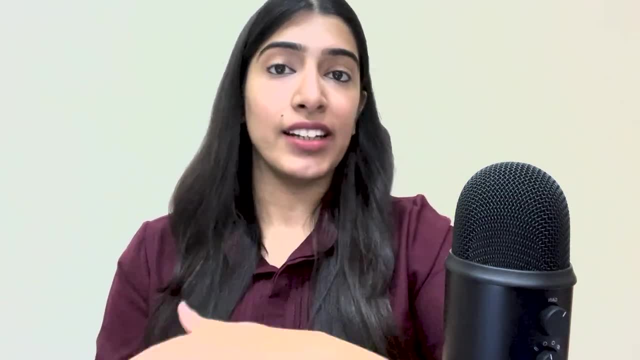 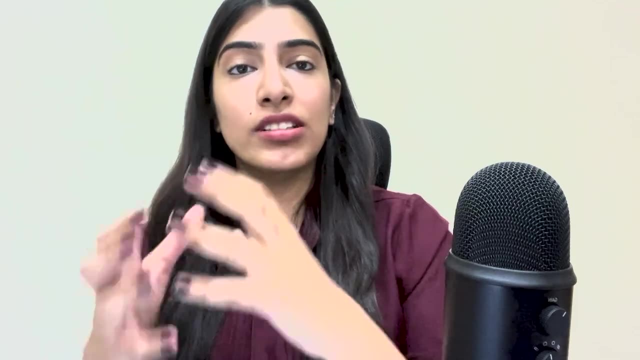 a house. Now, house has some common things to build right. It has a lot of parts. For example, there are interiors, there are doors to do, there is a roof, there is the flooring right. So these are the common things that you will do in all kinds of houses. Now the 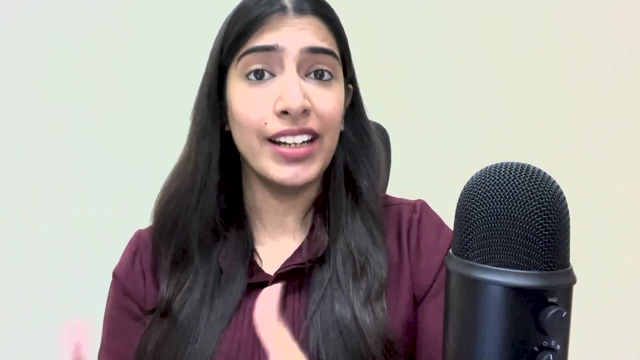 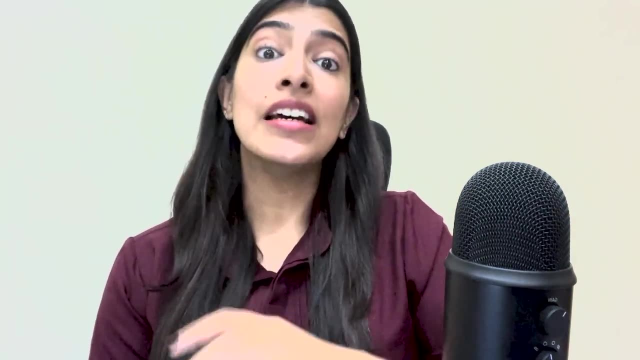 house can be an igloo house, Or it can be a house made up of wood. It doesn't matter Whatever the house is. these parts need to be built. Only they need to be configured according to the house type, right. Similarly, 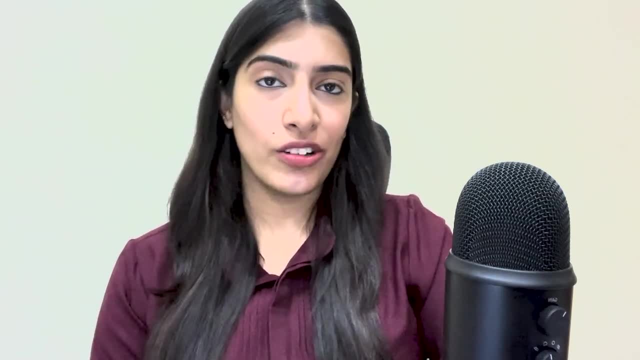 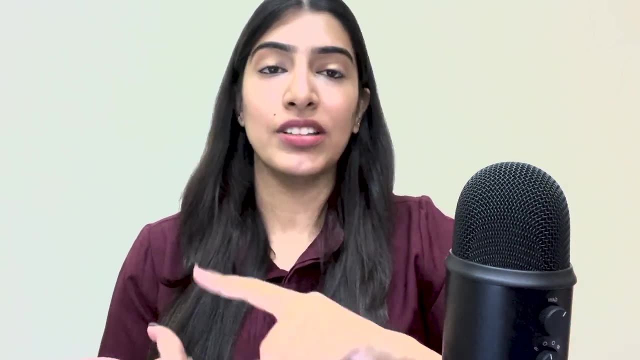 let me give you one more example. This is the example that we will be using for our book. okay, Now, when we have to build objects like desktop or a mobile right? So in a desktop, what all things are configurable? There is a monitor, there is a mouse, there is a keyboard. 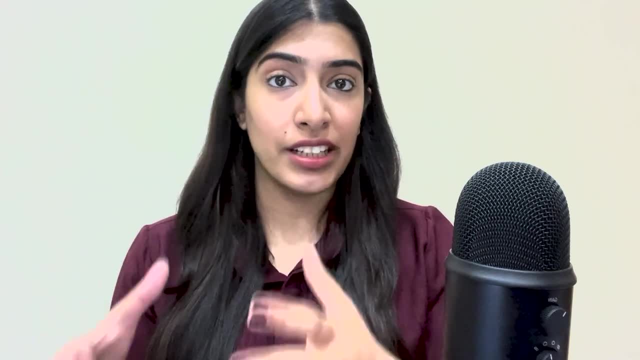 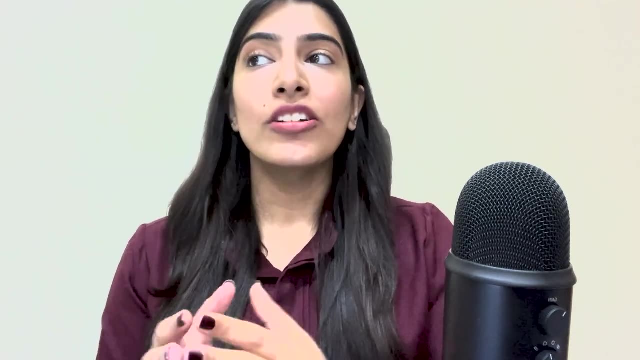 there is RAM, there is processor- All of these things are configurable, right, And it's a very complex object. You have to first build all of these parts and then create the house, Right, Or a desktop. Now, for example, I have to create an object, desktop. How will? 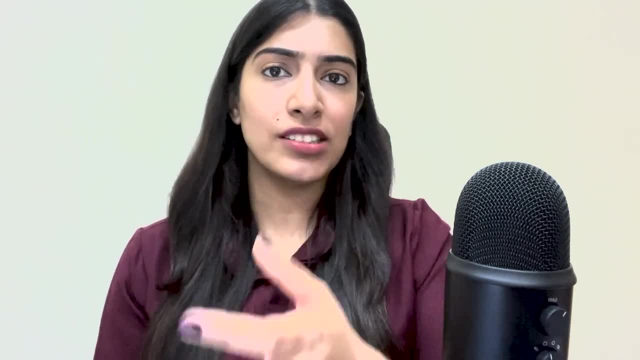 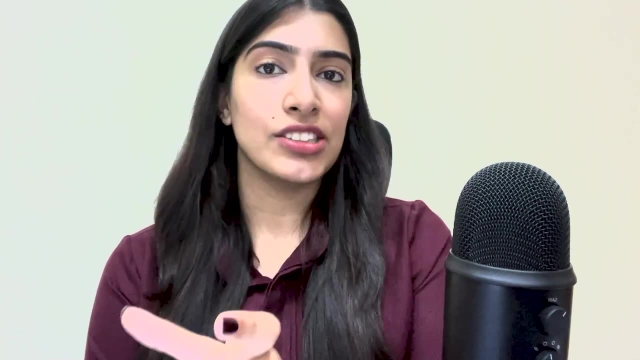 I do it. You will say: just give the constructor, just pass all of these parts after building them right Now. suppose tomorrow I have to change the type of RAM only, Or say in the constructor I don't want to give all the parts, I just want to give like four parts. 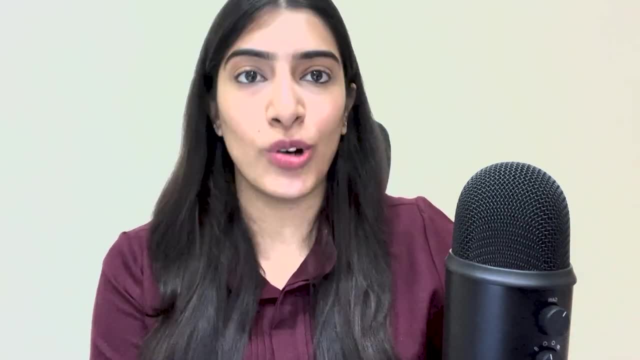 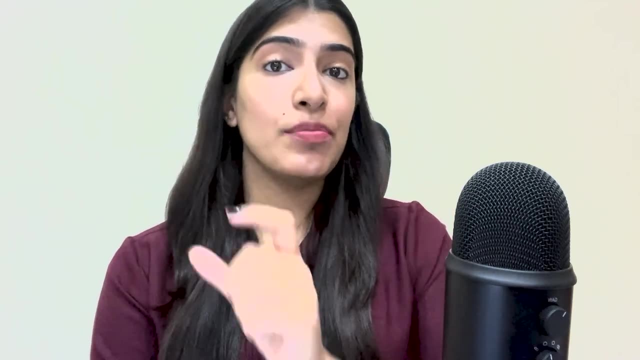 out of those 10 parts. The rest I will keep some default parts or I don't want to add that, For example, my laptop might have a touchscreen feature, right, But my desktop might not, So I might want to pass the type of touchscreen I am adding in the configuration. 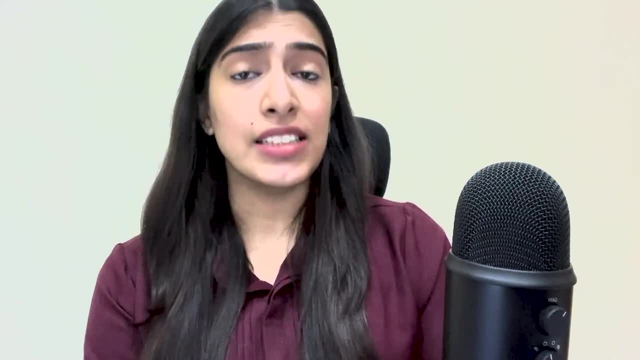 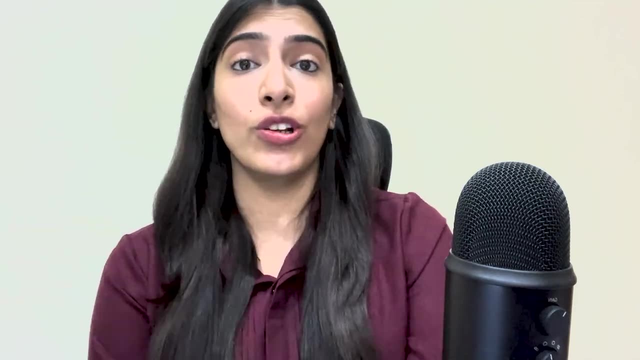 or I might not want to right. So, for all of these possibilities, are you going to write different constructors: One constructor with only monitor and RAM, another constructor with keyboard mouse, another constructor with all of these parameters, another constructor with touchscreen, another constructor without touchscreen. Are you going to write all of? 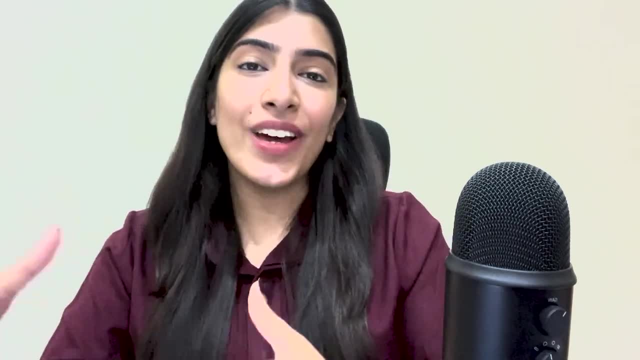 these? No right, That won't be flexible and readable. I know when I start writing the code some of you might go like: this is such a long code and I completely understand it can be overfilming, But I don't want to write all of these, So I am going to write all of. 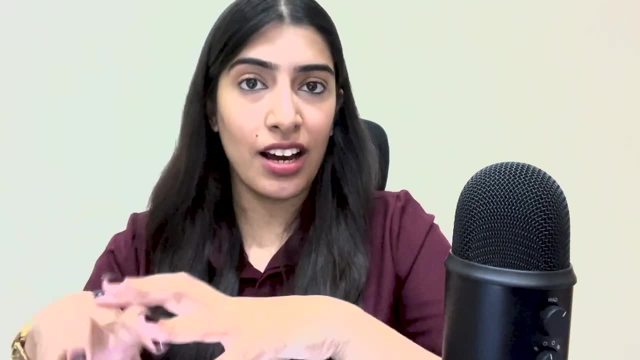 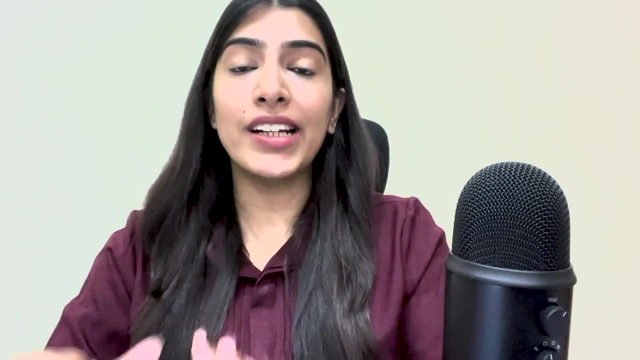 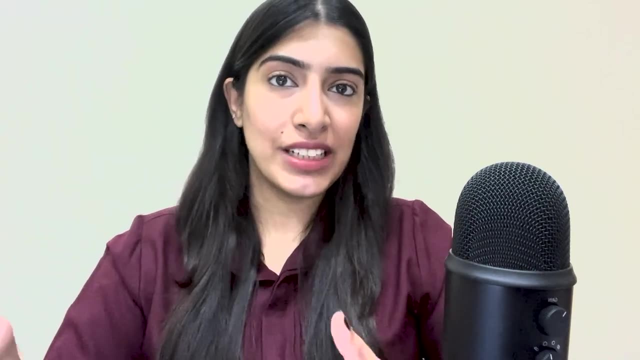 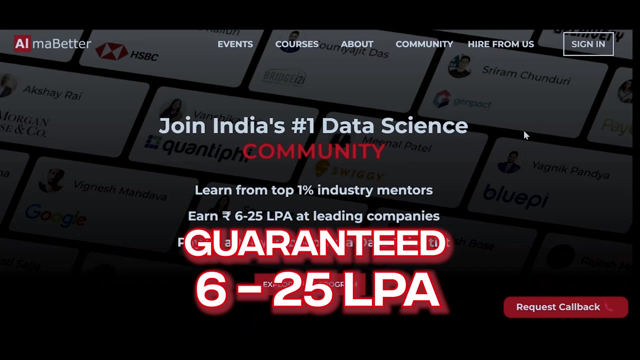 so much more readable and flexible. The code might be long, but it completely pays off because it's very well structured, flexible and ready. But before we go ahead- and I show you the diagram of the design pattern- let me tell you about the sponsor. Alma Better provides a placement guarantee of 625 LPA, So this: 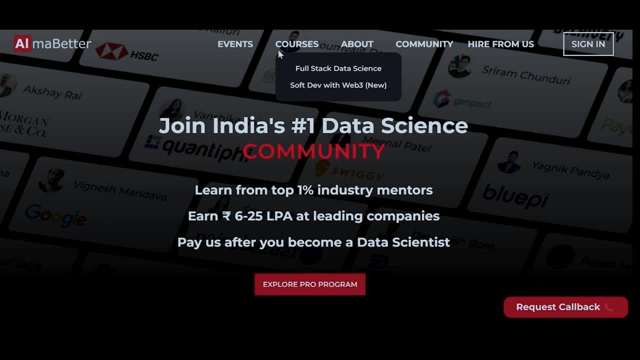 is not just a certification course but a well-designed curriculum, And I know that that you must be thinking that if they provide placement it must be costly. no, you will be surprised to hear that almabetta has an effective cost of inr0. how they work on the pay after: 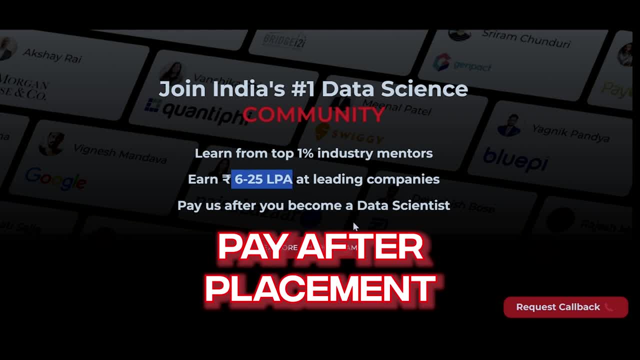 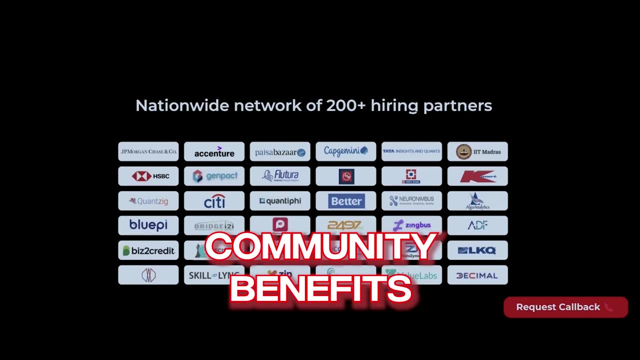 placement bundle, that is, they get you a job and then you pay them a part of a monthly salary for a fixed duration. they have a built premium network and community of working professionals, such as senior data scientists, ml, engineers, etc. 200 plus hiring partners, alumni and students you get to. 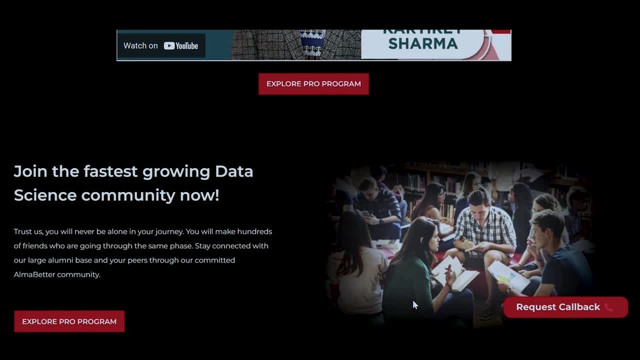 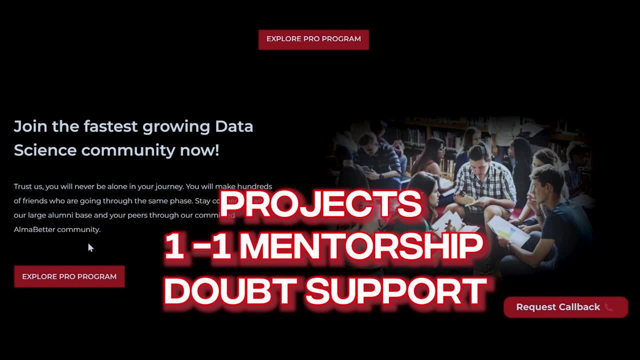 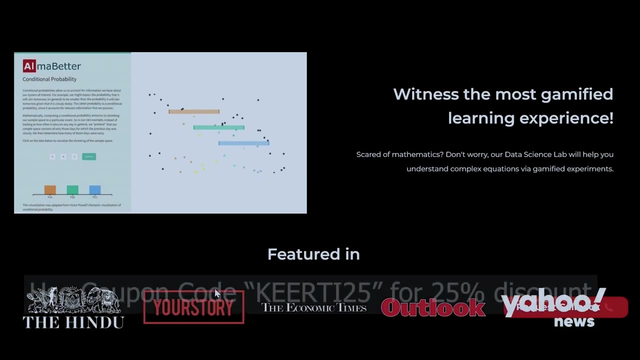 interact with them, get new opportunities as well as industry insights. almabetta's curriculum includes capstone projects, personalized one-on-one mentorship, doubt solving sessions, visual elements and gamification of concepts. you can also choose between live classes or self-placed learning. so go, check out the link in the description and don't forget to use the coupon code kirti25 to. 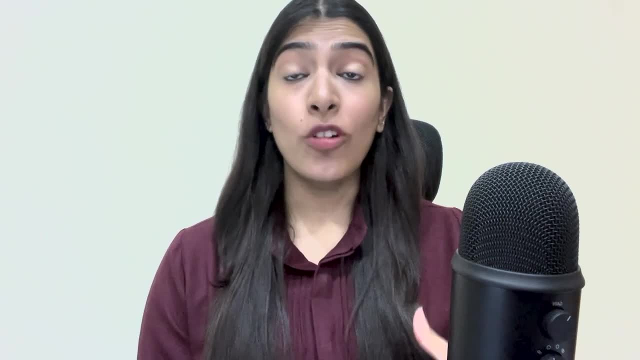 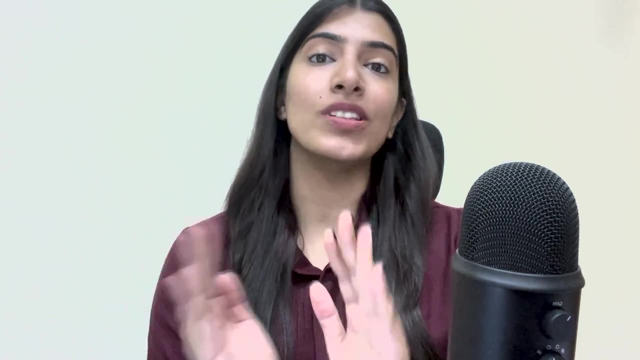 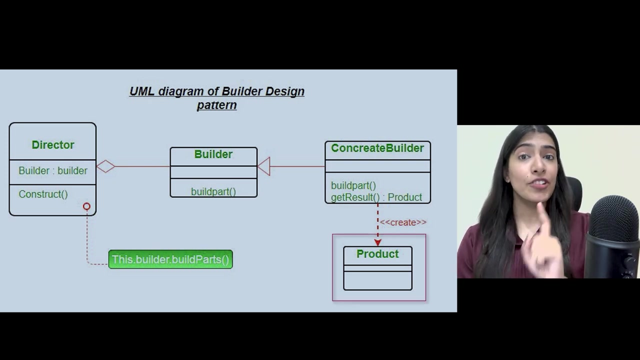 get 25% off on the course. now let's understand this diagram of build a design pattern and let's see the parts of it. if you understand this diagram, you have understood the entire design pattern, and then we just have to see the code. okay, so our builder design pattern has basically four parts to it. the first part is the product. 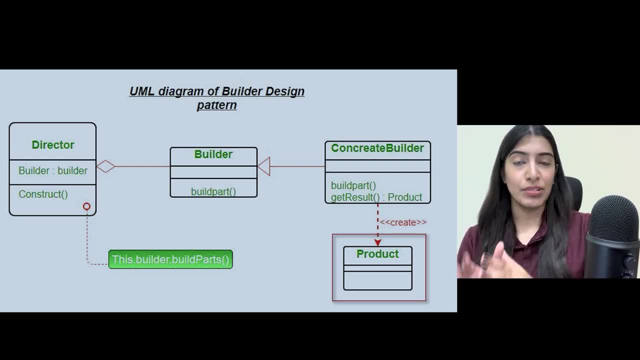 for the complex object that we are going to create, right in our example that we are going to take. the object that we are going to create is going to be a desktop. right now, there is going to be a builder corresponding to the product, which will be a desktop builder in our case. so our desktop builder. 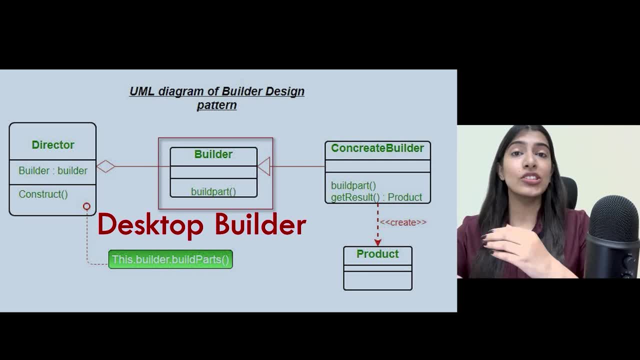 is basically an interface. it's going to be an abstract class which is going to tell: okay, these are functions, have to be integrated in this class, which is going to be the object that we are going be implemented by the concrete builders. i know, let me explain it to you. so there was a desktop. 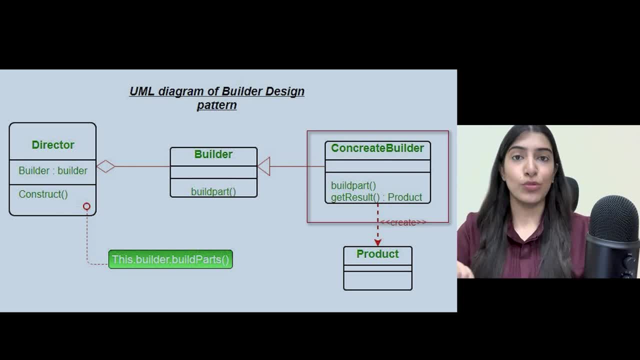 builder. now there are going to be two types of desktops that we are going to build. there is going to be a dell desktop and there is going to be an hpp desktop. okay, now, both of them will have their own configurations, their own type of monitor, their own type of keyboard and stuff. right now, our 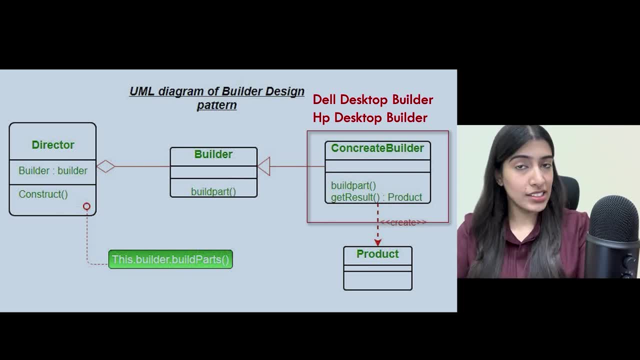 concrete builders, that is, the dell desktop builder and the hp desktop builder. these will have to implement the functions that are written in the interface. right, that is the desktop builder. now it will be like: build monitor, build desktop, build keyboard. now, both of these concrete builders- the dell desktop builder and the hp desktop builder- these will actually do the building. okay, they will. 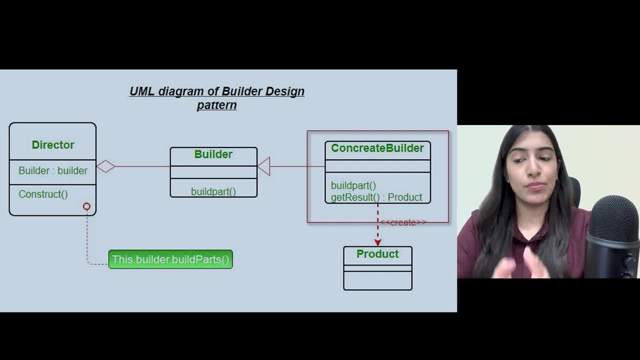 build their own type of mouse, they will their own type of keyboard and they are going to build. okay, the desktop builder is going to tell, okay, you have to build this, this. this concrete builders will actually use the configured monitor, the configured keyboard and actually build. so we have seen three parts till now. there is the product, which is desktop. 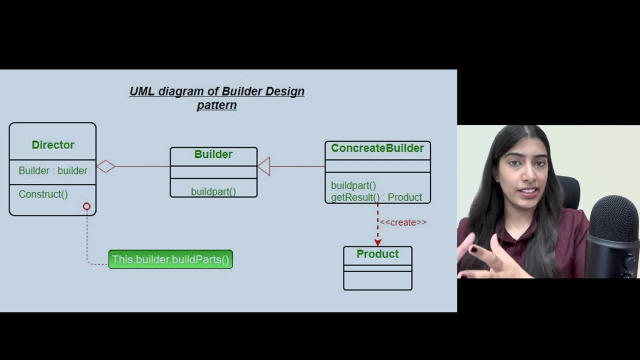 in our case, there is the builder interface, which will be the desktop builder interface in our case, and then there will be concrete builders which will implement the functions in the desktop builder. these concrete builders, in our case, will be dell desktop builder and hpp desktop. these three paths are clear. now the fourth component in our builder design pattern is a. 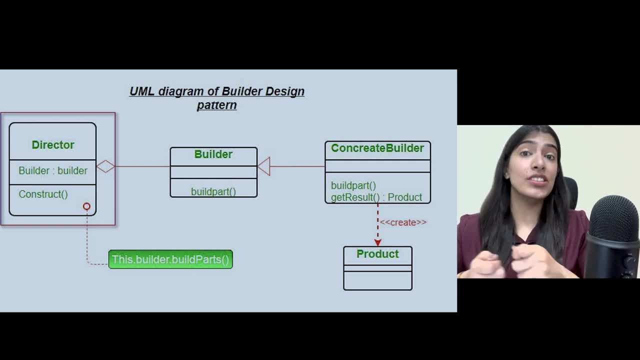 director, so director is responsible for actual generation of the product. it tells that all these steps will be followed to finally generate the product, the process towards it. so it will say: build the monitor first build the keyboard or the motherboard and then do this, this, this. so it will 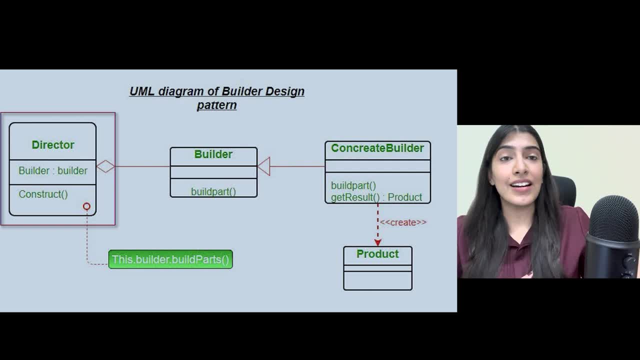 take care of the entire process. for example, when building a house, our civil engineer is going to be the director. it will tell you know what do this, this, this? then we will do those steps one by one. or, in case of building a desktop, the person who is building the desktop will be the director. 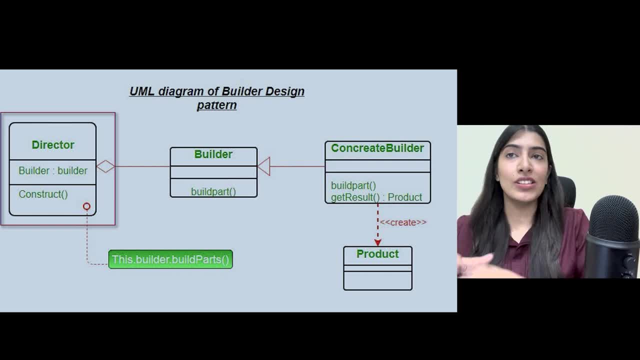 now, strictly speaking, some people implement the directors, or some people they actually call the client or the person who is using the builder design pattern itself as the director. so strictly speaking, you can actually call this component as optional, because the same code can be written in main itself and then our main actually becomes a direct. but to properly explain, 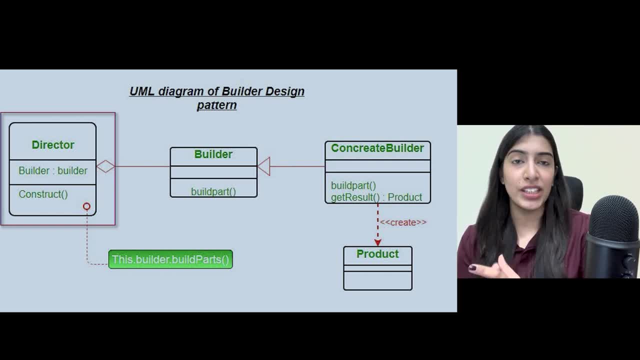 it to you. i'm going to write the code in a separate director component and i'm going to explain you that how it could have been written in the main inside. okay, so now let's get to our code and let's write these four components and see how the code works. again, guys, if it is confusing, it will be. 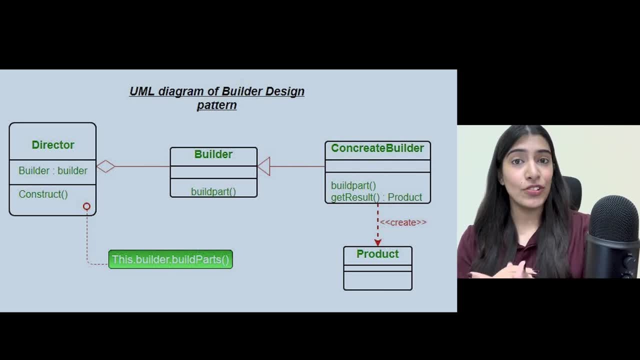 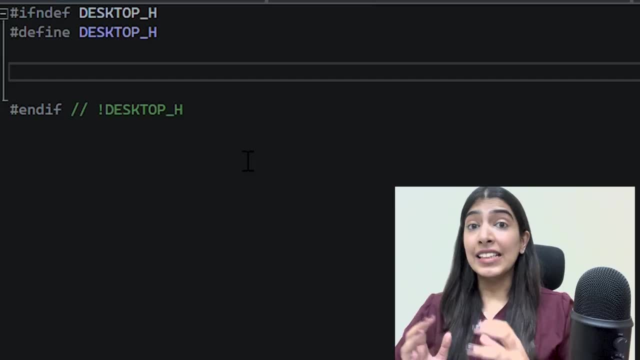 clear: just stay with me, stay patient. it can be confusing, but it will be clear. just stay with me, stay patient. but it will be clear in the end and our code will be super flexible, super readable. let's get started with the code. let's start writing some code now and let's get started. 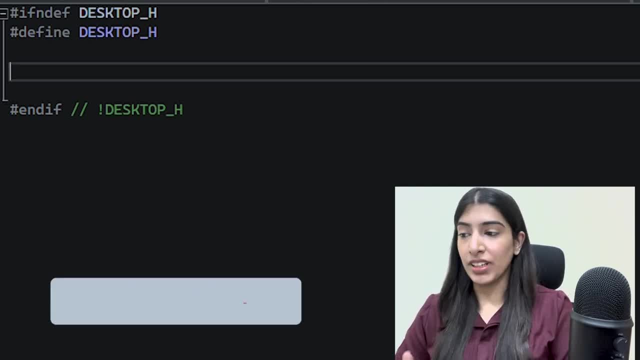 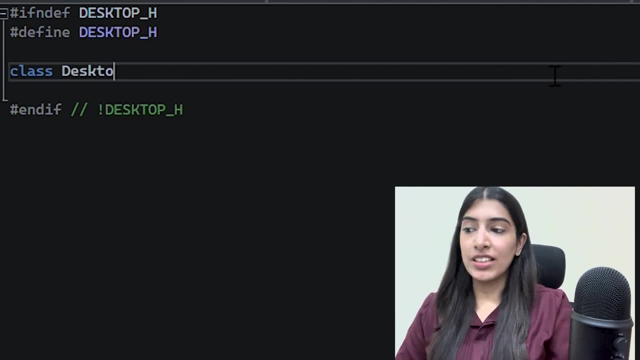 with writing a product which, in our case, will be a desktop right. so this is the desktop header file. in this, what am i going to do? i'm going to write a class desktop and in this, what? all things will be there, all the parts of the desktop will be there. so we're going to build a mouse, a keyboard. 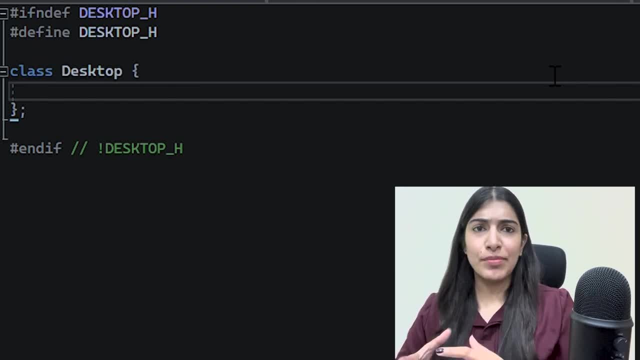 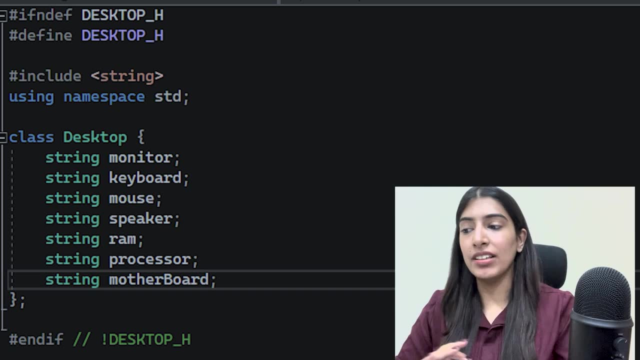 ram, a processor, all of these things will be there. so let me add that quickly. okay, give me a second. i have added all the parts of the products. for now i have given all of them as strings to keep things simple. otherwise these all can also be different. objects like monitor can be an object. 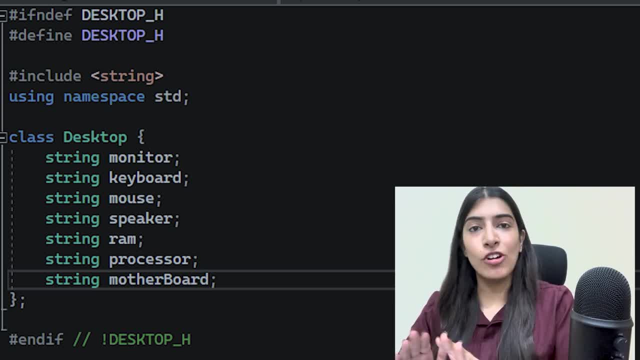 keyboard can be an object, mouse can be an object, and so on. but for now, for simplicity, i've made all of them as strings, right. what else do we need in our class desktop? so we have these parts of the desktop, but we also need to set these paths right, because these are all private paths. so we need 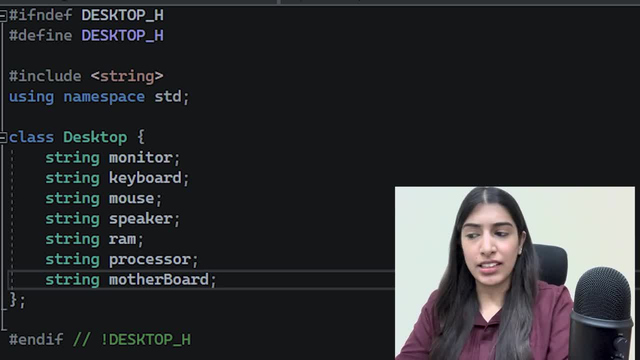 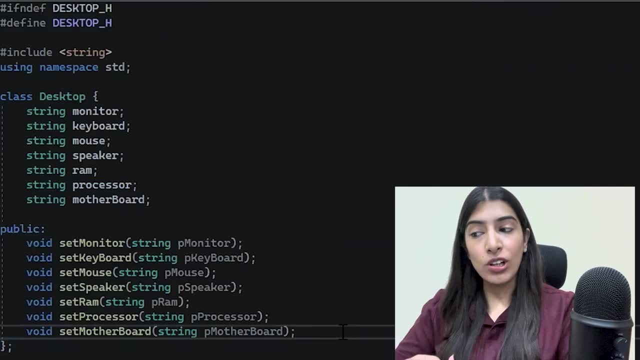 setters for these paths. so i'm just going to quickly add public settings so those setters can be called by anyone. okay, we are going to see who's going to call them. now you can see i have added setters for all the parts of the desktop. right, we? i'm going to add one. 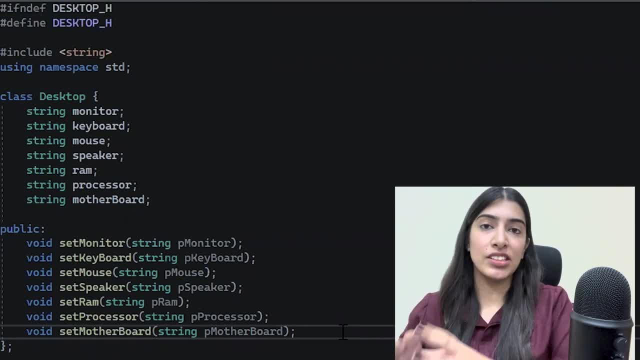 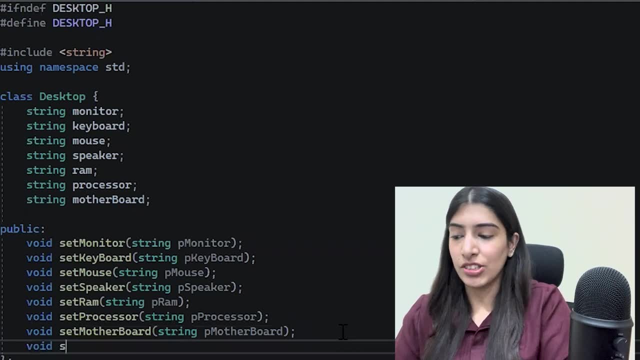 more function which will be just show specs, so that will be just to show the output after we have built the desktop. that, okay, the paths that i have added are correct. okay, so i'm going to add another function which is going to be called show specs of the desktop. okay, so this is our. 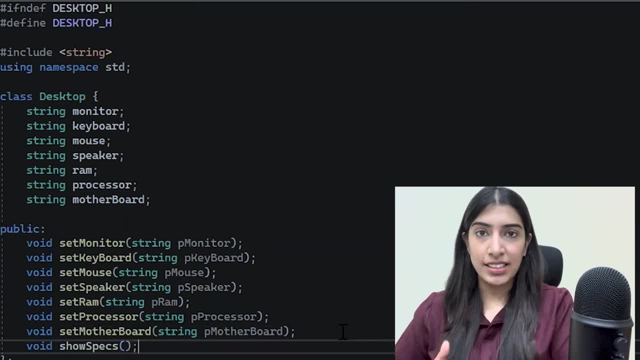 product, that is, the desktop header file. right, i have written some setters and this: obviously, these setters have to be written, right, they have to be defined. so the cpp file. let me just quickly, quickly, write these setters and let me show them to you. as you can see, i've written all the setters. 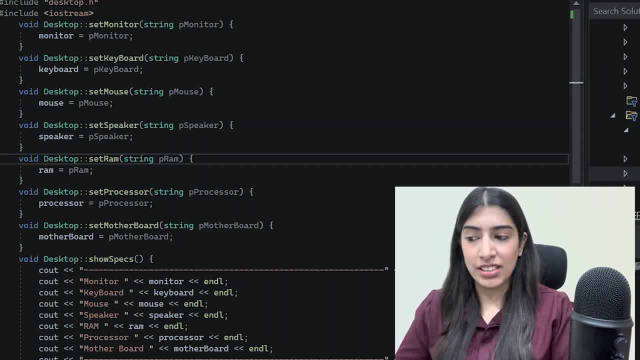 so i'm setting monitor, keyboard, mouse, speaker, ram, processor and the motherboard, and then i have written the show specs function in which i'm just going to output that, okay, this is the monitor, this is the keyboard, this is the mouse, and so on. so we are done with writing the product class, that is. 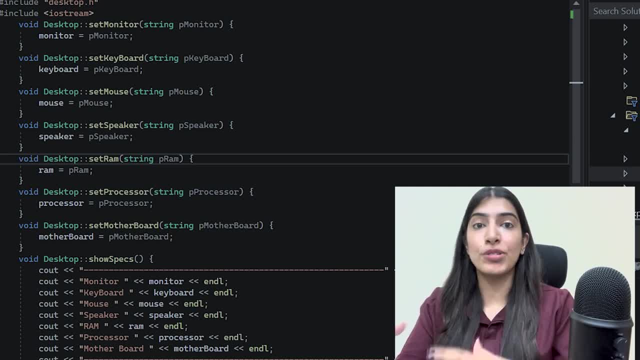 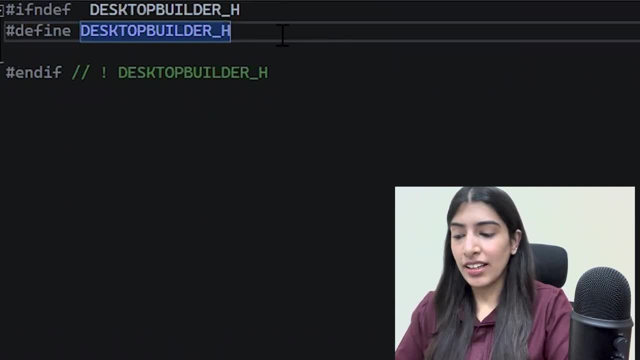 the first component- desktop class- right? what was the second component, the builder? so we are now going to write a desktop builder class. this is the desktop builder header file. so what is going to be this? there is going to be a class- desktop builder- right? so i'm writing that class right now. 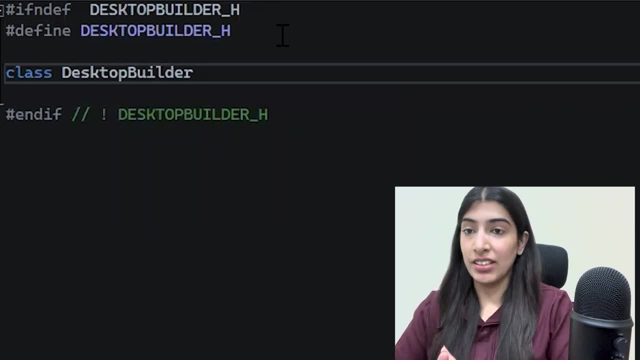 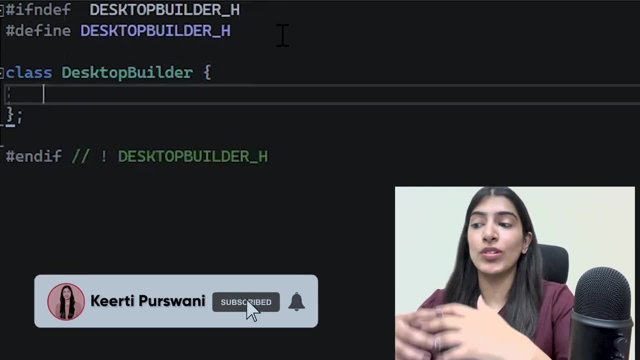 and what is going to be in this builder. we need the product inside this builder, right, so we will define a product over here. also, keep in mind that our product needs to be accessed by all the concrete builders which will be inherited by this desktop builder, right, and that's why i'm going to 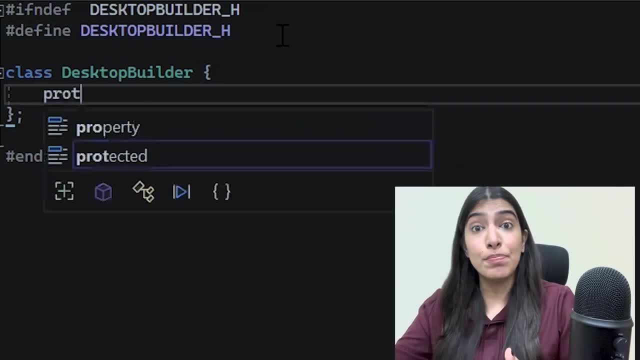 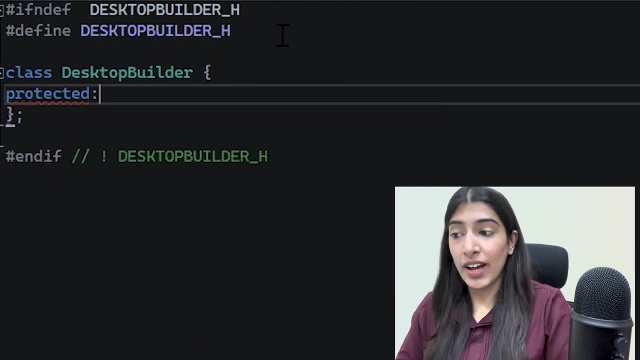 make our product inside this, which will be a desktop in the protected environment. so i'm going to add a protected section and i'm going to add the product inside this. but to add the product, we also need to include the desktop class in this. so i'm going to include desktoph. 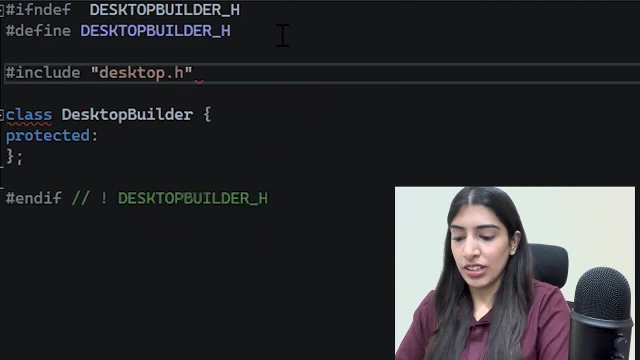 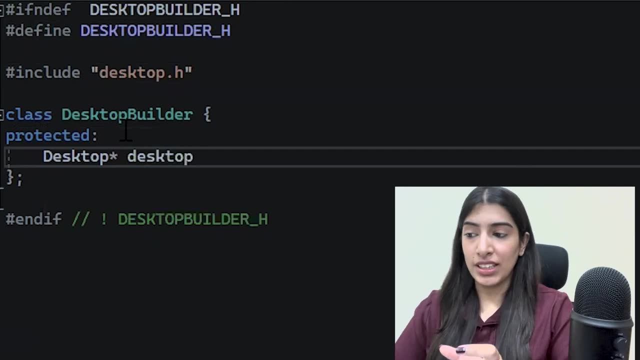 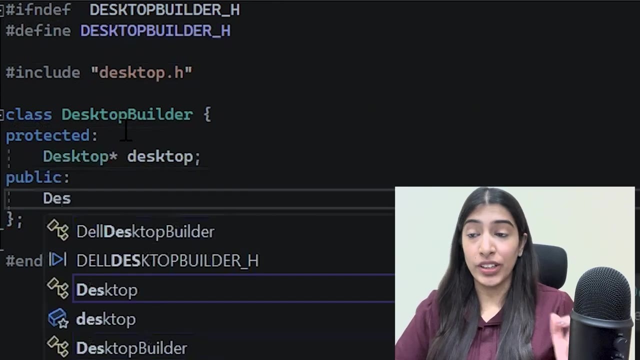 right now, since i've included it, i can have the product over here. so desktop is here now. what we are going to do is, in the constructor of the desktop builder itself, we are going to initialize this desktop so as soon as a builder is created, a product is created corresponding to it. 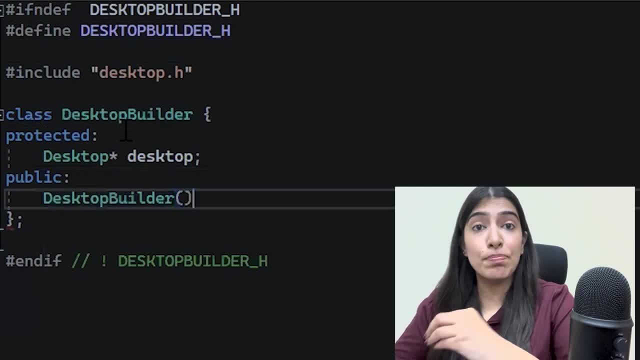 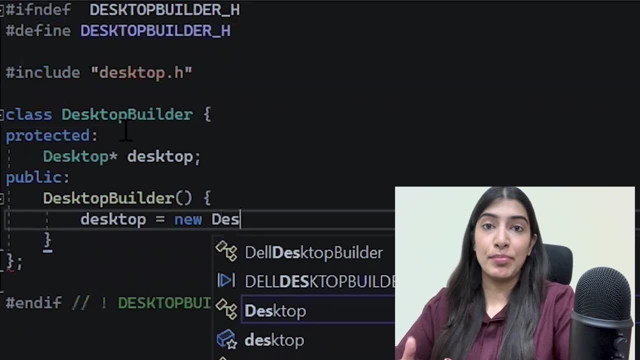 but this is a simple product. this is a simple desktop. none of the parts have been built or none of the parts have been configured right, so we need to add all of those parts which will be implemented by our concrete builders. so now let me add those parts. as you can see, i made all of my 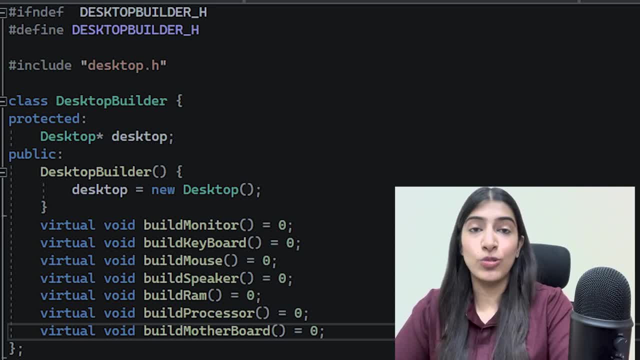 builder functions as pure virtual functions, because i've written virtual, void and equal to zero, which means all the concrete builders, that is, all the classes that will inherit from this desktop builder, have to implement these functions, so they have to build them on the keyboard or mouse. so our desktop can't be just as it is. we need to add these paths to it. that is why we need to add the parts which are already there. 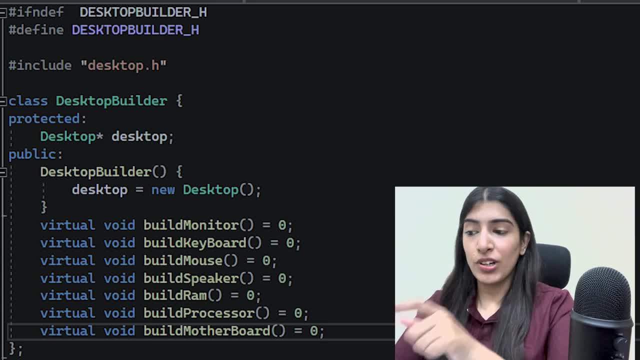 what i have done right now. okay, now the desktop product is over here, right, so i can actually write a getter of the product over here also. now some people, while implementing the builder design pattern, what they might do is add the getters in the concrete builders like in their desktop builder. 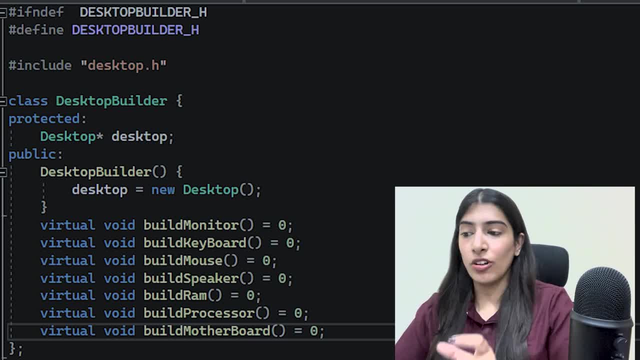 and in hp desktop builder they might write the getter of the desktop there instead of writing it over here. that is not wrong thing to do, but in our case what is happening? we are building a desktop product. only right because the type of product that will be developed by both the dell. 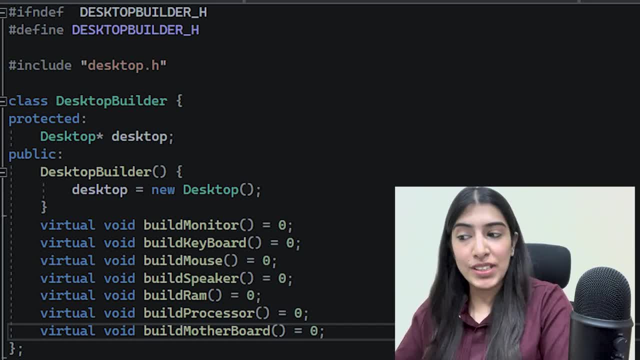 desktop builder and the hp desktop builder will be desktop itself. that is why we can have the getter over here. but for example, we were building, say, car and a scooter. right, they might have like different, uh, return types, like one might be a car type and one may be a scooter type. 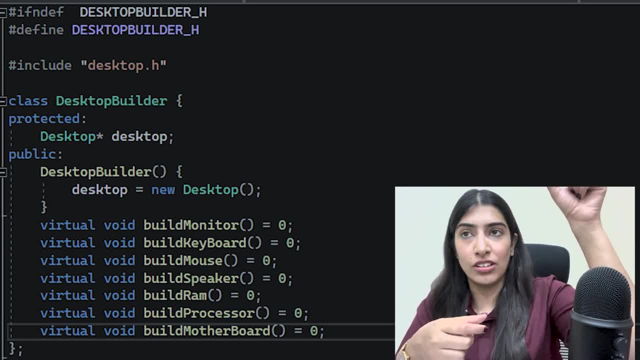 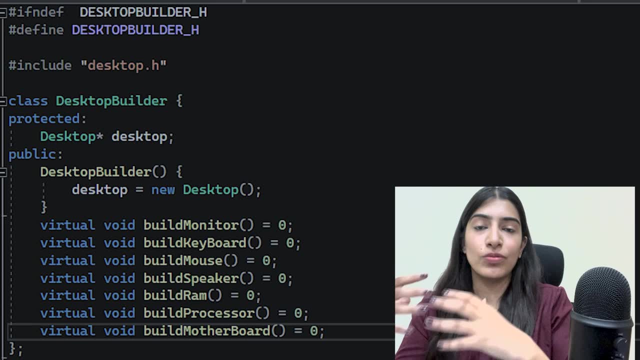 ideally what would have, what should happen is that they both are also inheriting from vehicle and we are returning a vehicle. so in that case also we could have like a vehicle getter is self. but suppose we don't have that and our getters have to be separate. in that case what? 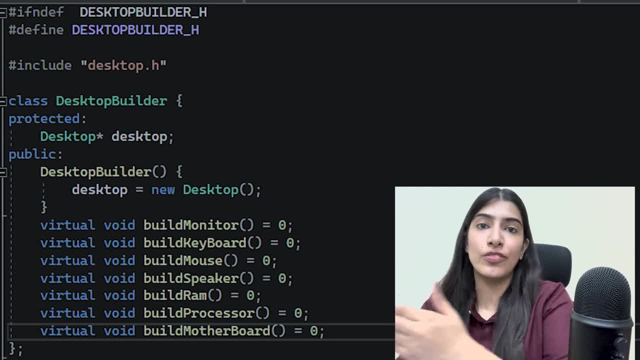 we can do is write the getters in the concrete builders instead of writing it over here now. these are the minute details that can actually confuse people, that you know where things are supposed to go in builder design pattern in which component is supposed to go, but don't mind into going into. 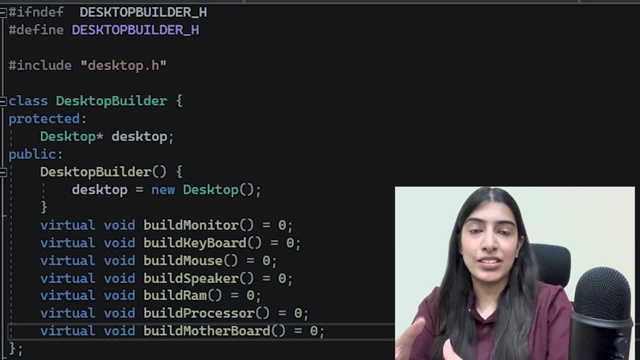 so much detail because the way people implement builder design pattern might be a bit different here and there. this part is not that straight. so we can actually write getter with a getter with a getter. we can actually write getter with a getter, so that's why we can do that. so let's see. 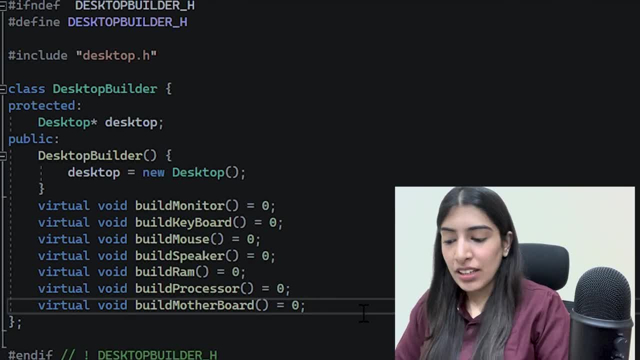 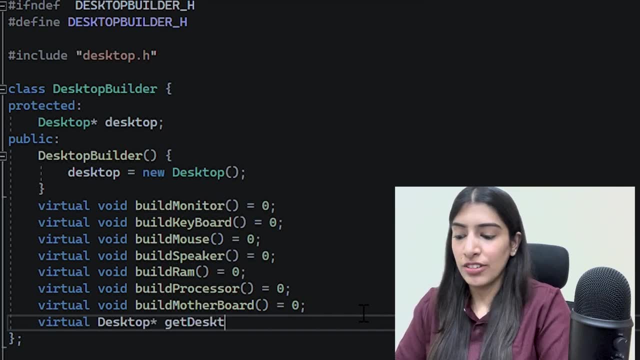 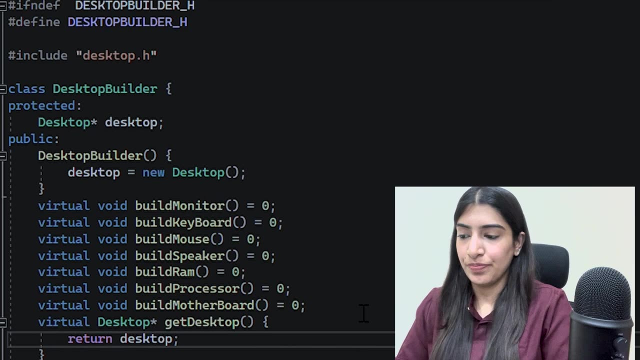 the concrete builder itself. i hope you have got the point. i am making it virtual so that, in case it is required to override it, it is possible, and i am returning a desktop pointer. i am going to call the function as get desktop and i am going to return our desktop from here. we are already. 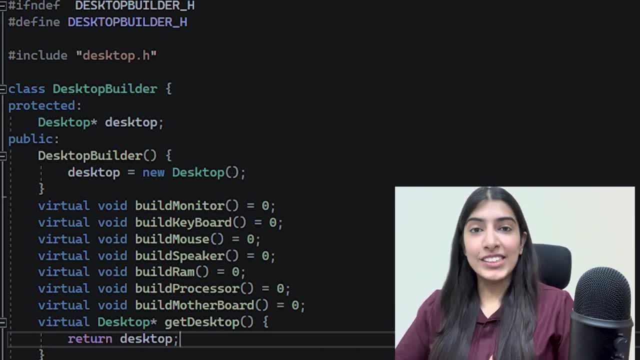 done with our second component, which is the desktop builder. now let's finally get to our third component, which is the concrete builder. so we are going to finally write the dell desktop builder and the hp desktop builder. it's very simple. all we have to do is really just implement. 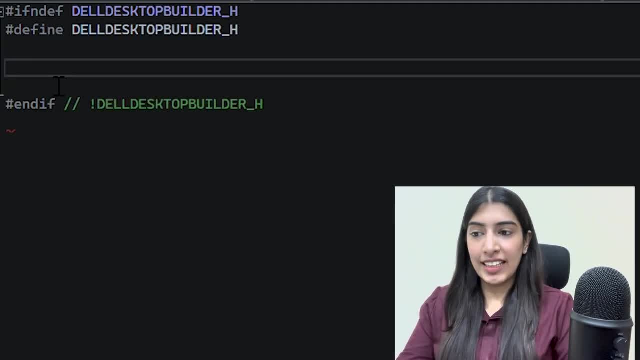 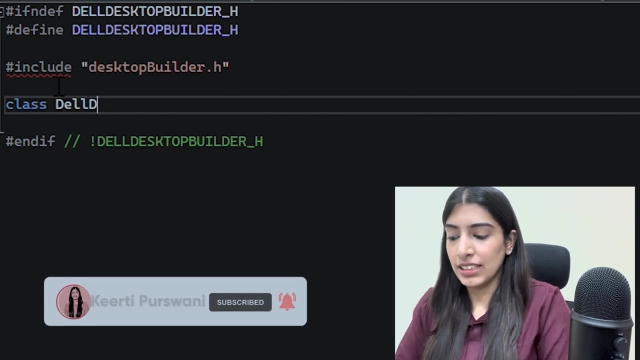 these pure virtual functions. so let's do that quickly. this is the dell desktop header file. in this i need to inherit from the desktop builder, right? so i need to include desktop builder and once i have done that, i can actually write my class, which i am going to call as dell desktop. 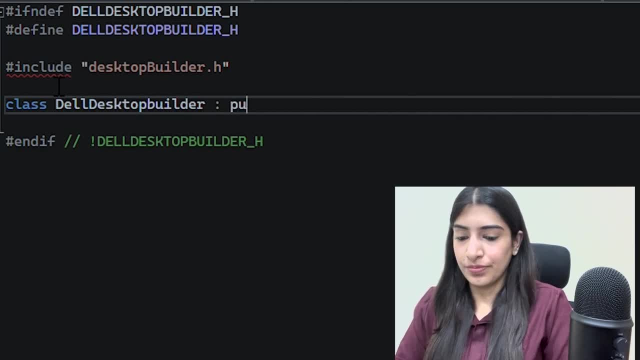 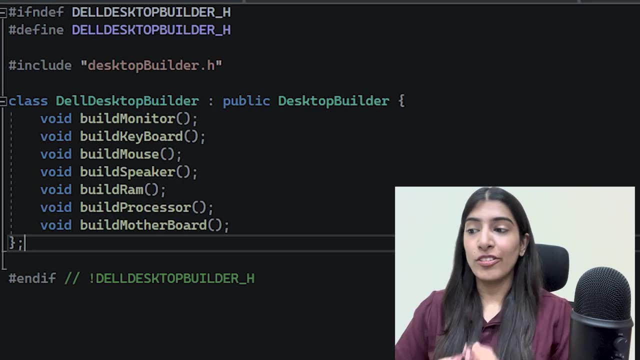 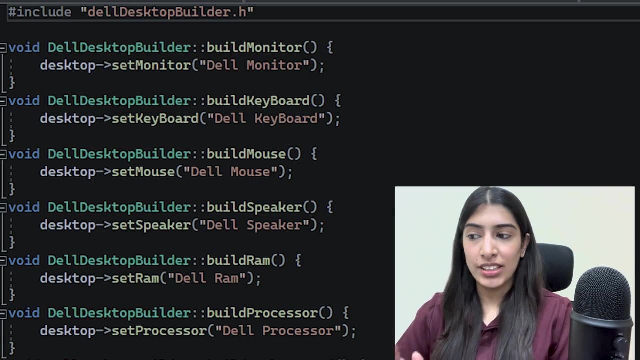 builder and i am going to inherit it from the desktop builder, and i have added all the functions that were there in the desktop builder over here, and i obviously need to write the functions, the cpp file also. so, as you can see, i have included the header file in the cpp file. and what have i done? i have just set all of them right, so right. 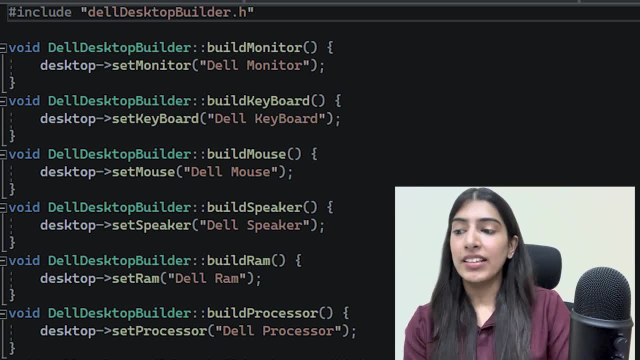 now i was setting strings only. so i have just written: dell monitor, dell keyboard, dell mouse- there's speaker- dell ram del processor and so on. right, so these are strings itself, but in real life, what would happen is that i would actually build the paths over here and i would 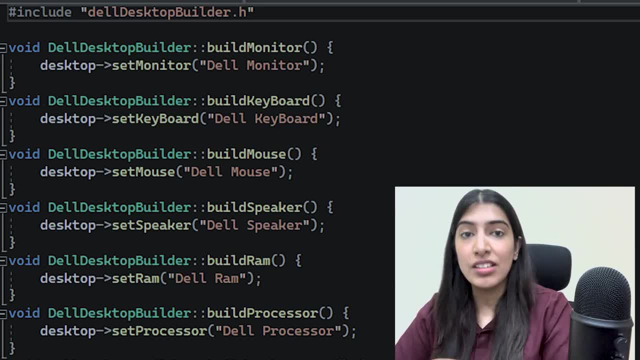 configure and configure them. so if i am building a dell monitor, i would configure over here that i am building a dell monitor, right, and in the hp desktop builder i would actually configure the monitor over here right. so my concrete builders are for the configuration part. so here i have. 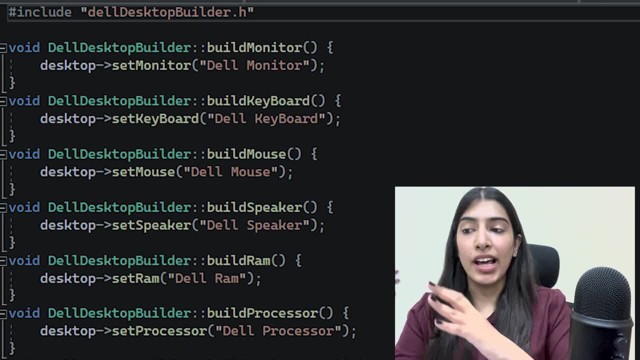 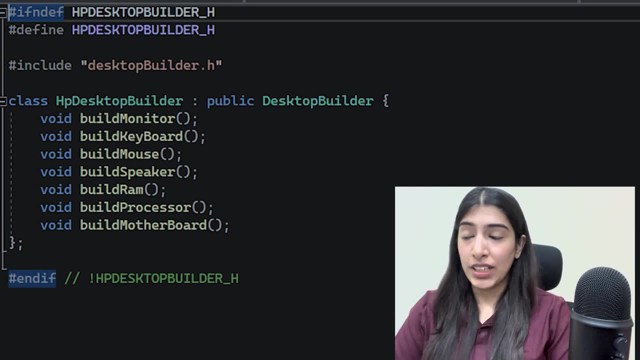 just passed the strings to keep the example simple, but i'm going to do the same thing in the hp desktop builder to really show you that how it looks. this is my hp desktop builder header file and this is exactly same as the dell desktop header file. i have just written the cpp file and 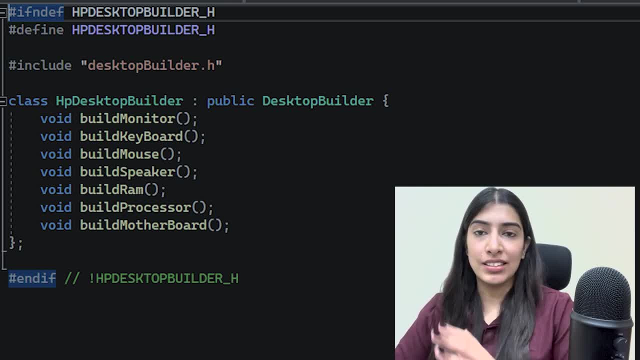 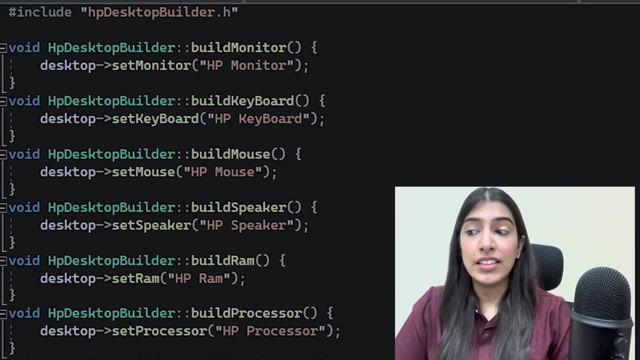 written all the functions as it is. i'm going to do a similar thing in the cpp file, as i did in the dell desktop builder, and this is how my hp desktop builder cpp file looks. as you can see here, i have configured as hp monitor, hp mouse, hp keyboard right. the strings i passed are different from: 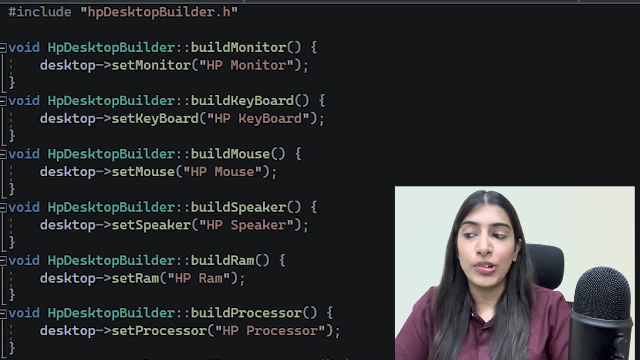 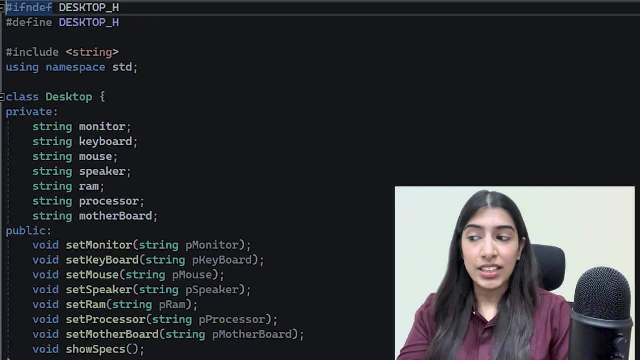 the dell one. there i was writing dell monitor, dell keyboard. here i have written hp keyboard, hp mouse, right. so here i have configured it in the, in the concrete builder. so we are done with the important of builder design and let's quickly revise it. first, we made the class desktop, which was our 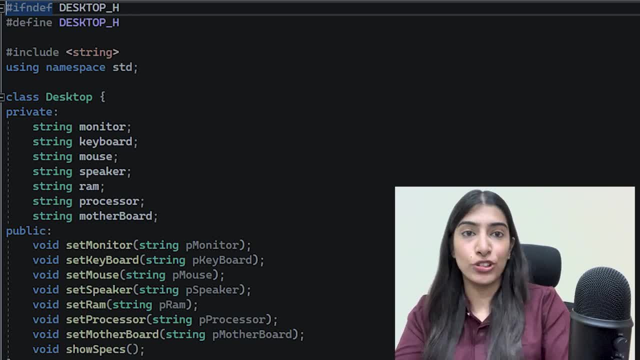 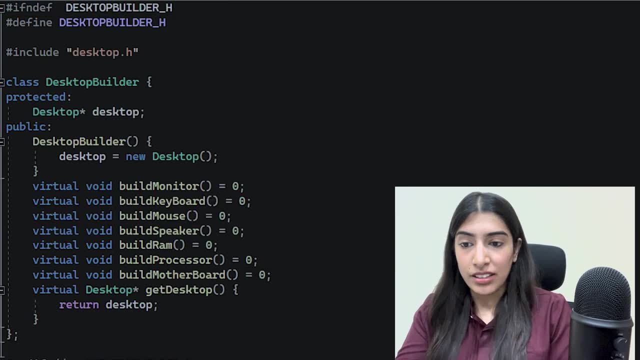 product. in this we just wrote that, okay, what all paths are going to be there in the desktop, okay, and we wrote the setters for those, the cpp file. then we made a desktop builder. in this we just wrote pure virtual functions so that our concrete builders know that virtual functions have to be. 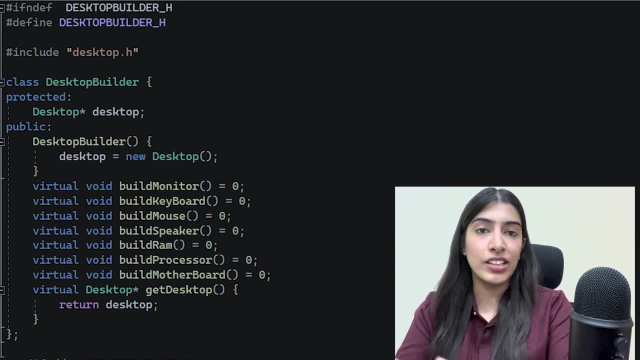 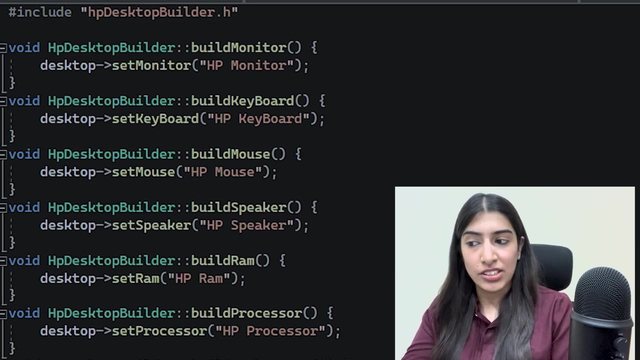 implemented and we wrote a getter over here that, okay, we need to return the product. in this and in the constructor we had initialized the product for that product. okay, so this was our desktop builder. then we wrote two concrete builders: one was the del desktop builder and one was the hp desktop builder. in both of these all we have 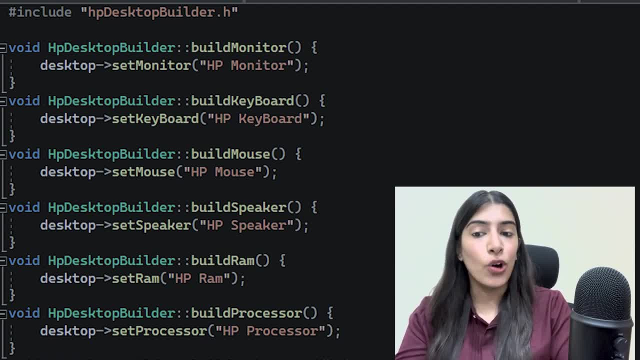 done is just implement the pure virtual functions that were there in the desktop builder and we have configured them accordingly: the cpp file. so in the del desktop builder we send dell monitor, and in the hp desktop builder we send hp monitor, and so on. now let's come to our 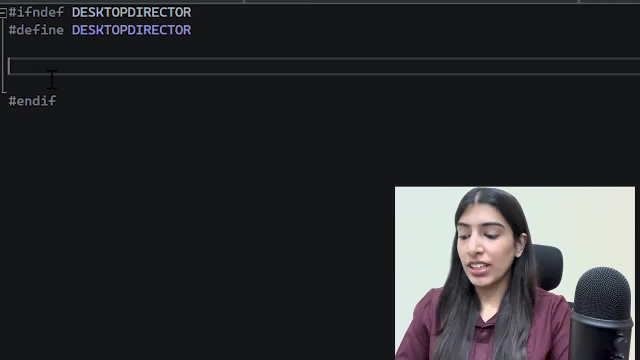 final fourth component, which is the director, are at our director component in this. what do we need to include the builder? right, so a builder will be sent to the director and a director will use the builder to create our product. okay, so we need to include our desktop builder in this. so let me add the desktop builder that i have done. 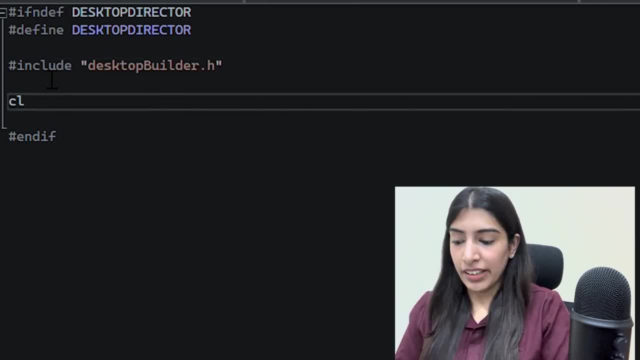 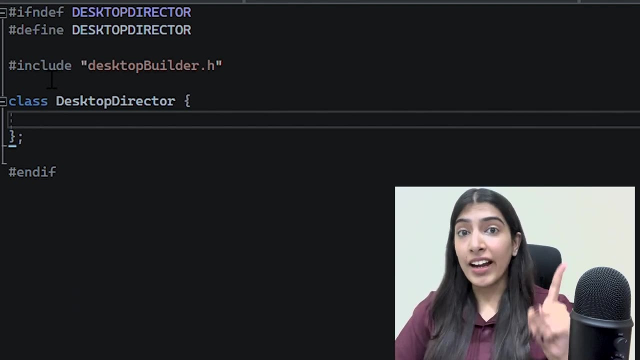 now i am going to write the class desktop director now in this director we need builder as a member. see in the builder there was product in director. there will be builder and director will use the builder to build the product right. again, to keep it very simple: a builder has product, a director. 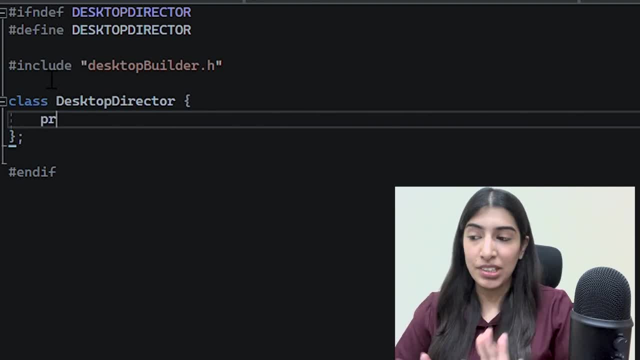 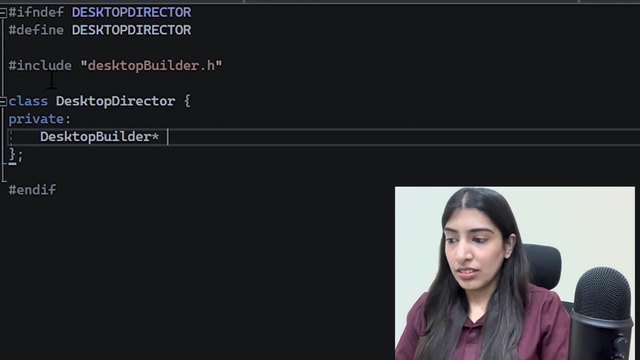 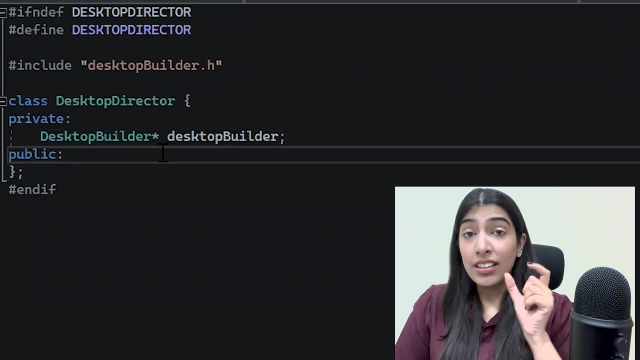 has builder which is going to use the builder to create the product simple. so we are going to add the builder member in the private section. so in the private section i have added desktop builder. so in the constructor of the desktop director, builder will be passed. i just have to. 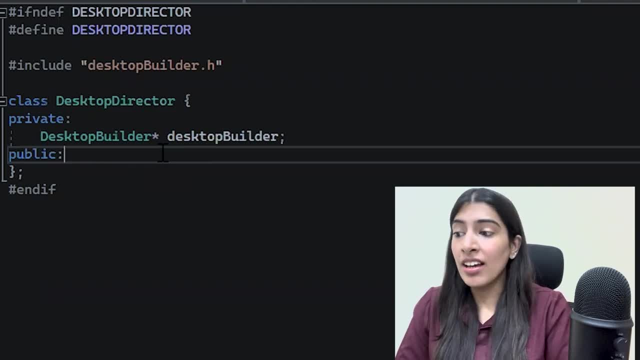 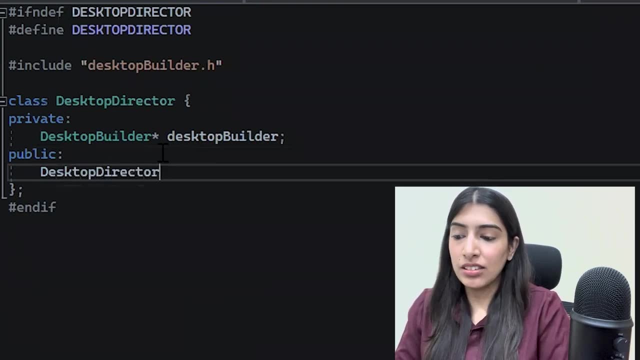 assign the member to that builder, right? so let's do that. i am going to write the constructor desktop director and it will be passed for desktop builder. so for a parameter, i'm just adding p, i'm going to call it desktop builder and i'm going to assign my 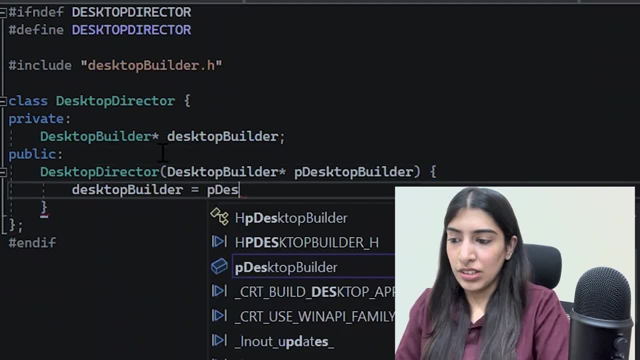 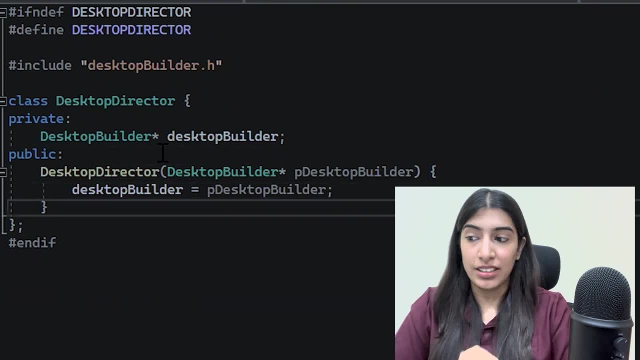 object: desktop builder as p desktop builder. now, what is the main function of the director? it tells: actually, let's build a product in that desktop director. it's going to direct the entire process. let's see how. so in this there is going to be a build desktop function which is going to return desktop. so we are going to write. 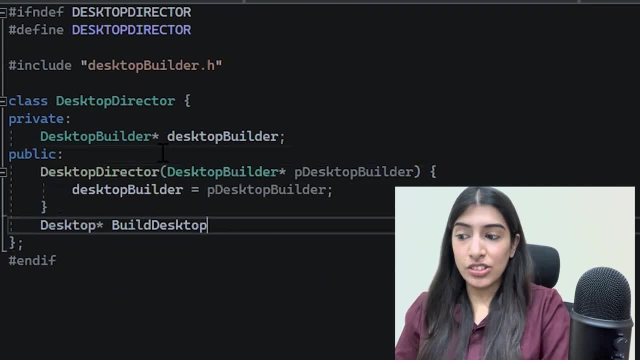 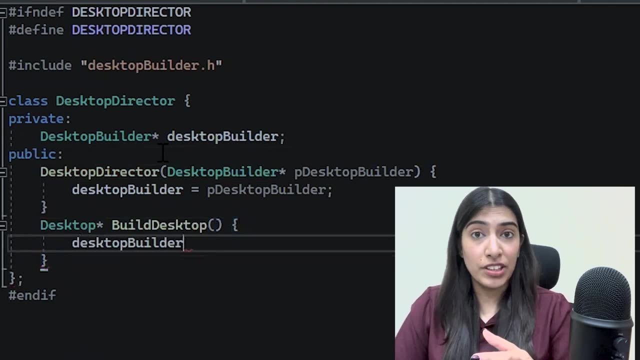 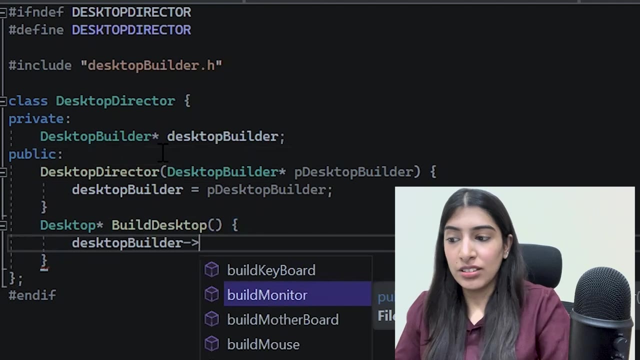 build desktop. so director is going to do the entire thing. right, it already has the desktop builder and this desktop builder already has all the bit fun. so now what I'm going to do is call those one by one and actually build that desktop. so what I'm going to do build monitor, then I'm going to do build. 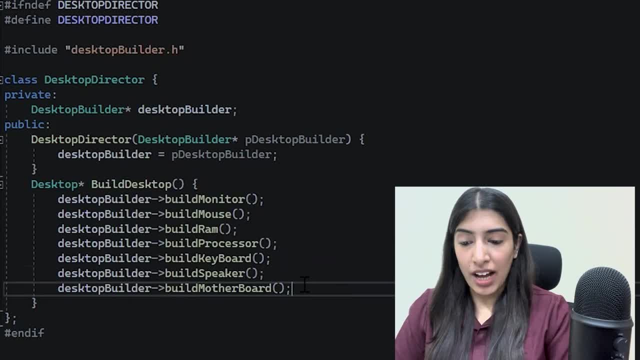 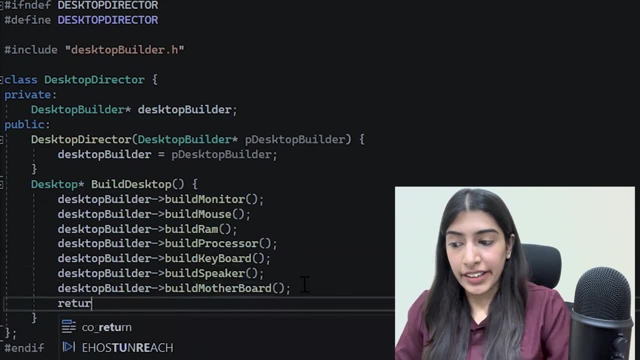 keyboard and similarly. I have built all the paths. and now, since in this function I'm returning desktop pointer, I am going to say the builder itself had a getter right, so desktop builder had get desktop and I am going to return the desktop. now see another point over here: in this function I am returning a. 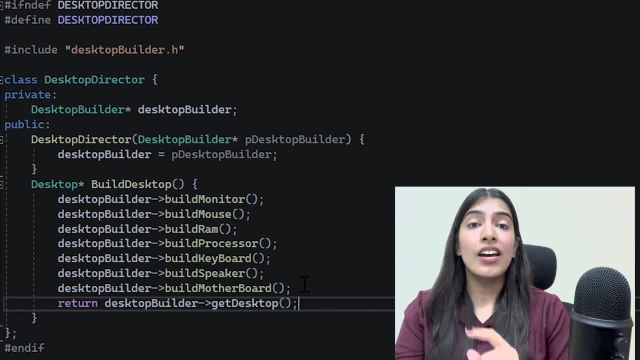 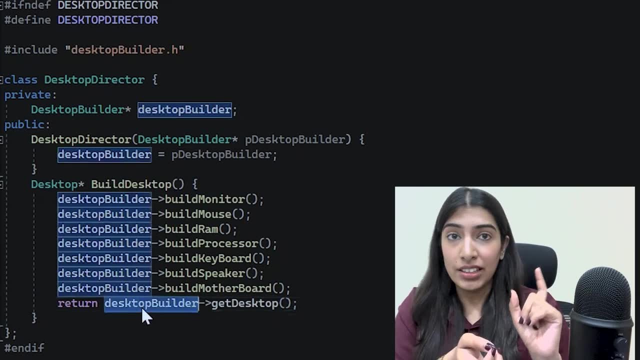 desktop pointer and I am calling a get desktop right. first thing I'm going to do is I'm going to call a get desktop and I'm going to call a get desktop and I'm going to notice over here is: I am calling the builders get itself right, the getter that we had written in the builder class, remember? 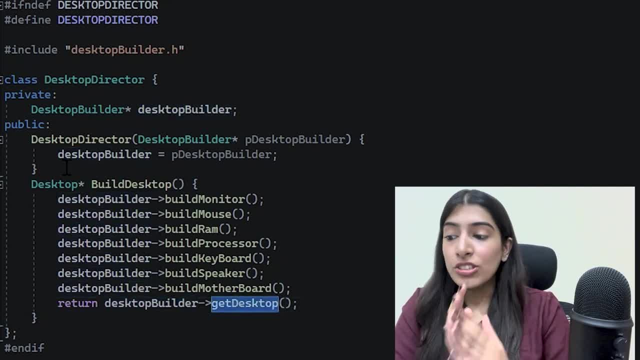 which I was telling that you could write now concrete builders also. so I am calling that getter over here to actually return that desktop pointer. what some people might do is use this function to just build and not return anything from here that you are building, and they might write a separate getter. 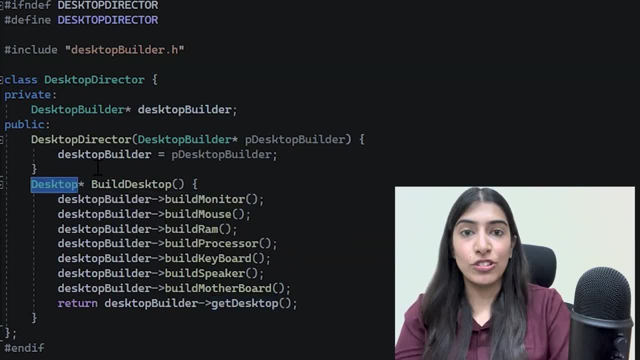 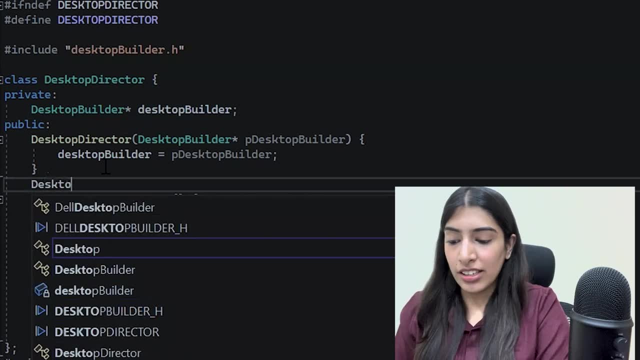 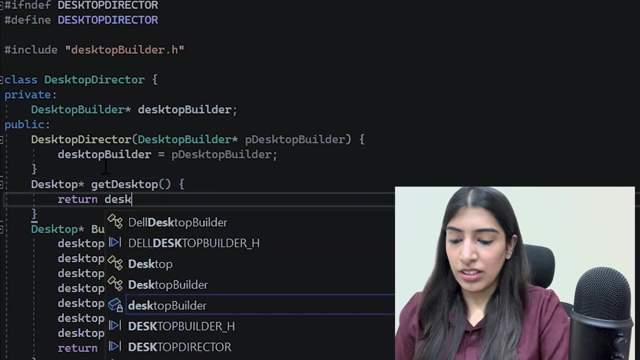 right. so I am just writing that getter also separately to show you that, how that can be done. so what I'm going to do is I'm going to return desktop. from that I'm going to say get desktop and I'm going to use my builders function to return the desktop. so desktop builder. 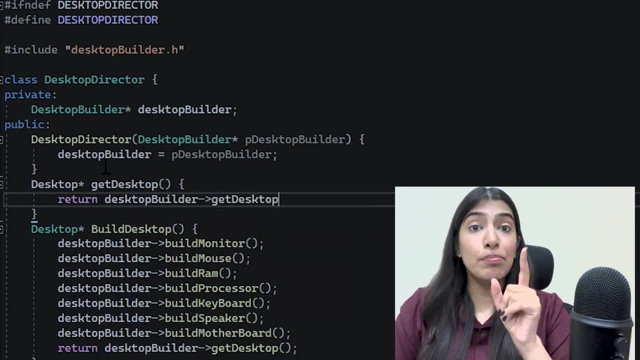 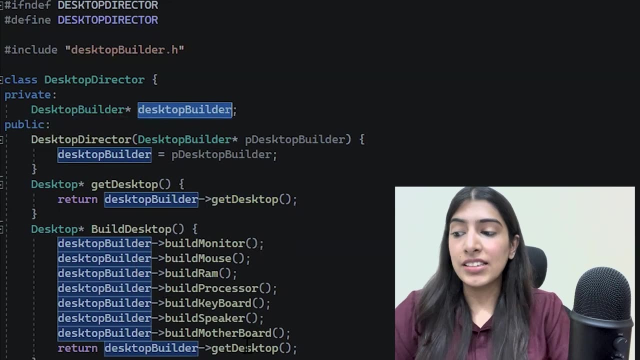 and get desktop. to again make it clear: our builder had a product and a builder had a getter of the product also. now our desktop director has the builder and now the director is using the builder to get the desktop and it is building the entire product through the processes. see, these processes are already written. 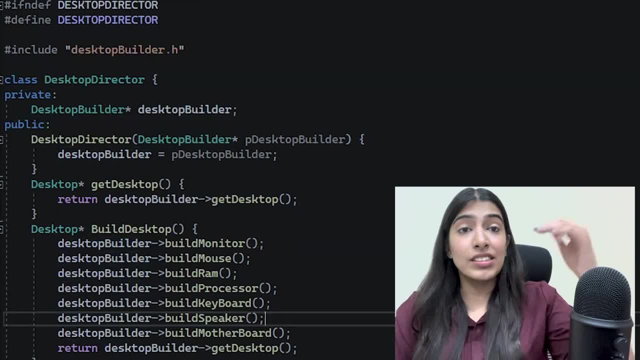 in the builder, but the only thing that director is doing is giving it a process. it is actually calling the build processes and building the things while building a house. also, what a civil engineer will do. he or she will tell that, okay, these are processes are to be followed. it will tell the builders and 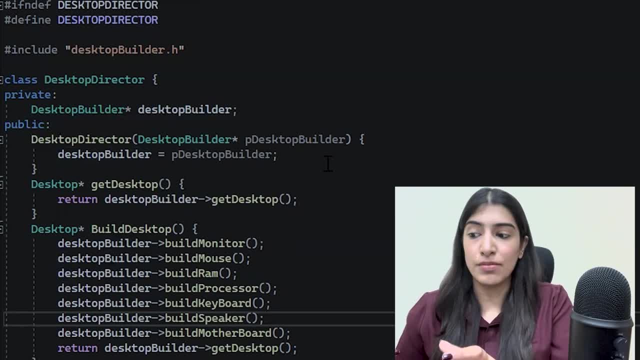 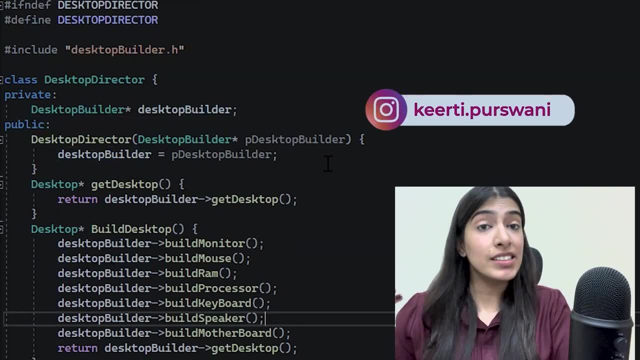 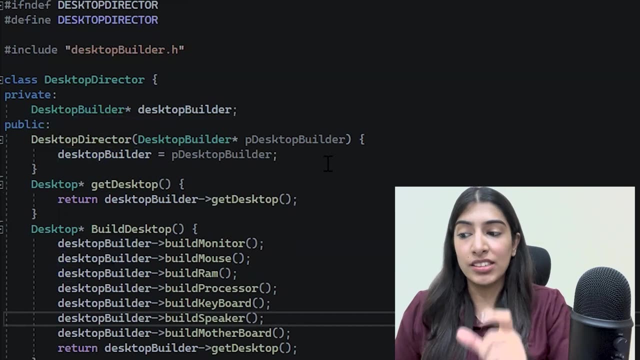 now builders will actually take care of the configuration part that I need to build a, what kind of a roof or what kind of flooring here. also, see, I have just passed desktop builder. now this desktop builder could be a del one or two, an hp1, it does not matter. what i am going to do is just pass the desktop builder and i'm going to 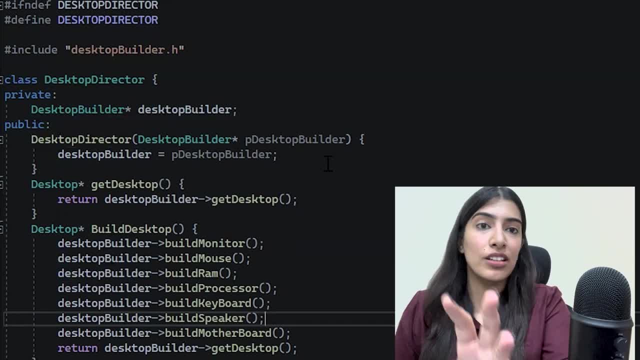 tell the builder that you add the configuration and then you build the monitor and you give me- and i'm just going to return the desktop right now- that we have written all the four components, let's finally see how our client can use our builder design pattern and how easy it will be. 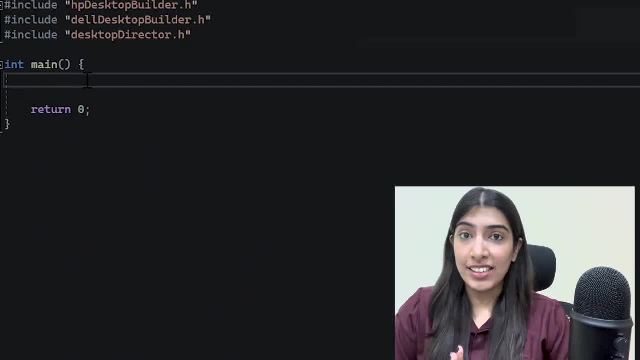 for our client to use it. this is the final part of understanding the design pattern. guys, you have actually understood everything. you just have to see how it works. this is the most interesting part of this right. as you can see, i have included the hp desktop builder and the del desktop builder. 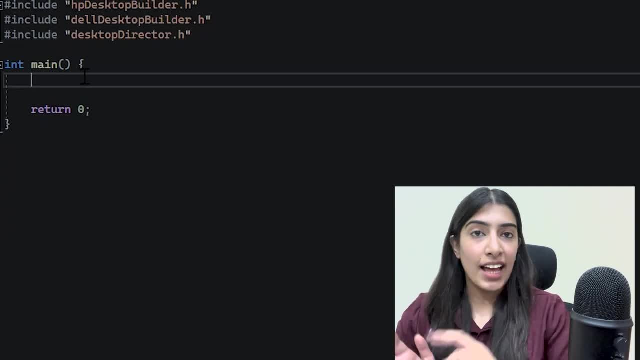 and i have added the desktop director, right. so let's actually write two forms, two types of builders, and let's write two directors who will be given these two different builders and actually build two different ones. let's do that. so let's first use hp desktop builder. 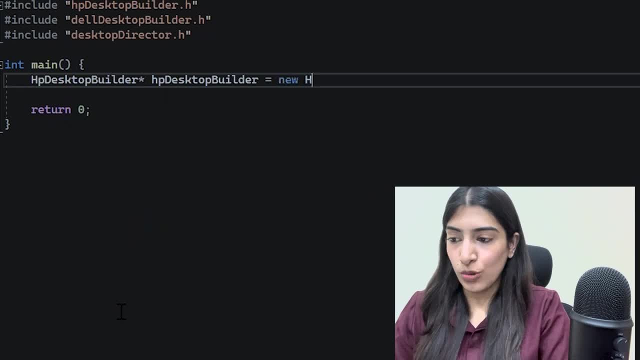 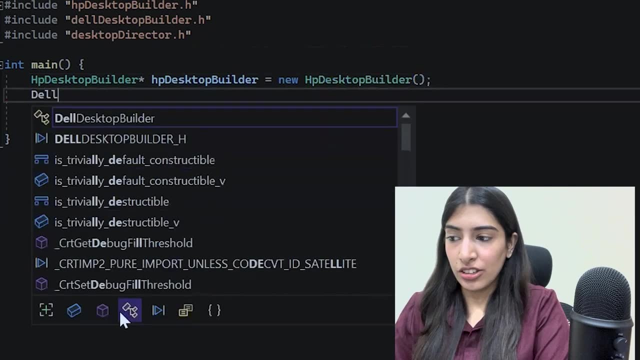 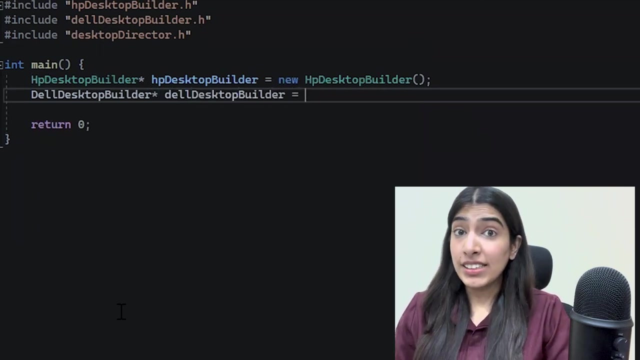 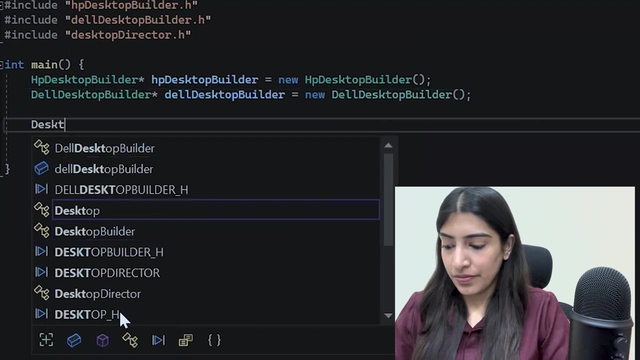 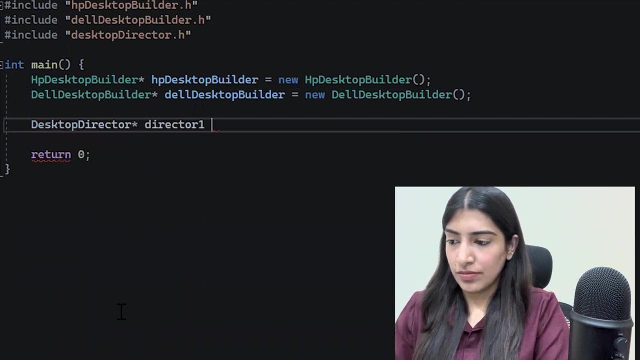 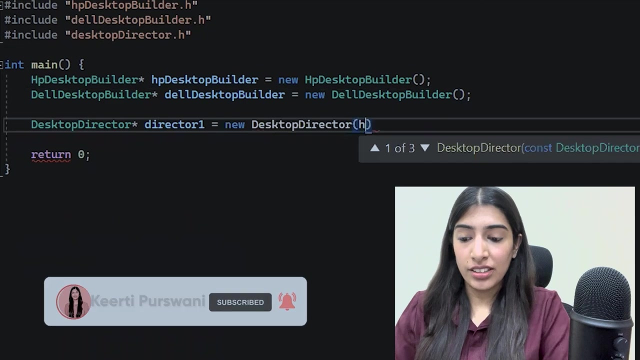 i'm going to create a new one and i'm similarly going to write a new del desktop builder. and now let's write two different directors and pass one of these builders to each of them. so let's write desktop director one. what were we passing in the desktop director? consider we were passing the builder right. 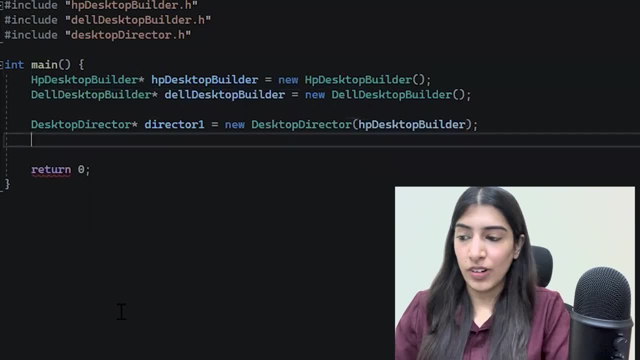 so we are going to actually pass the hp desktop builder in one and we are going to pass the del desktop builder in the other. now that we have two directors, our directors can actually build the desktop in our build desktop function that we have written in our director. we had actually, we were actually returning the desktop. 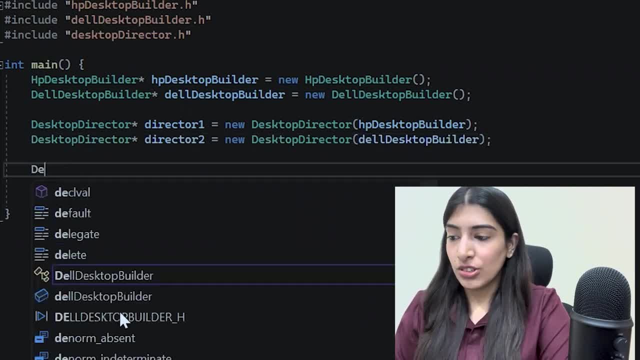 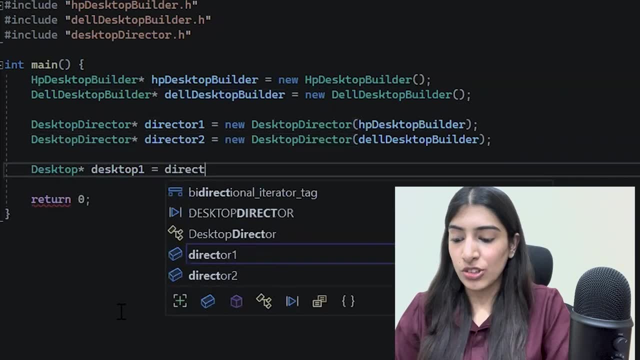 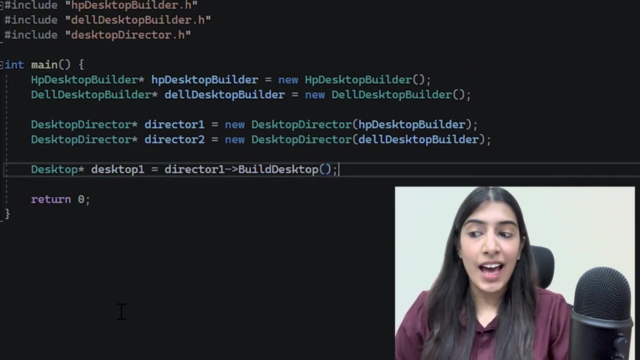 right, so we can actually return the desktop. so let's write desktop one and it's going to be returned from director one and it's going to do build desktop. so we don't need to pass anything over here, see, because director one already has the hp desktop builder, so it already knows that i have. 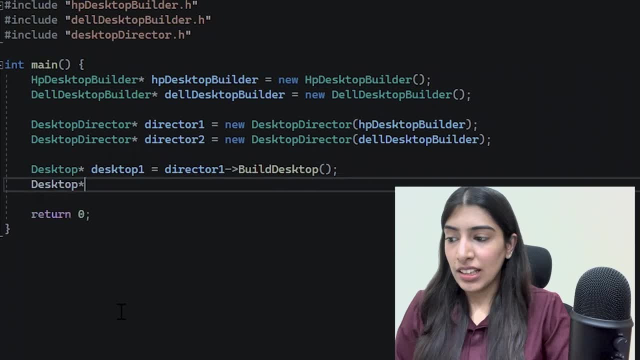 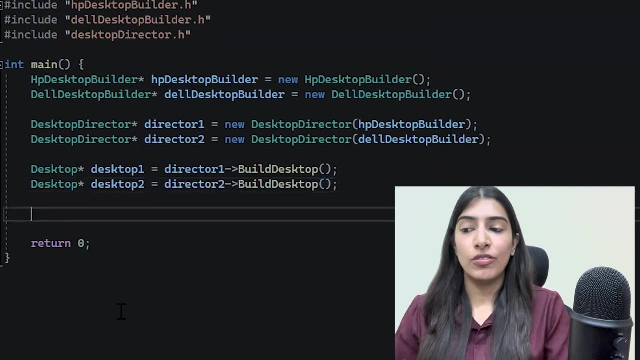 to build an hp desktop right. similarly, let me create one more desktop. so i'm creating desktop 2 and our director two is going to build this and since we have already passed the dell desktop builder to it, we don't need to tell it again. it already knows that. okay, this is my build. i'm going to build. 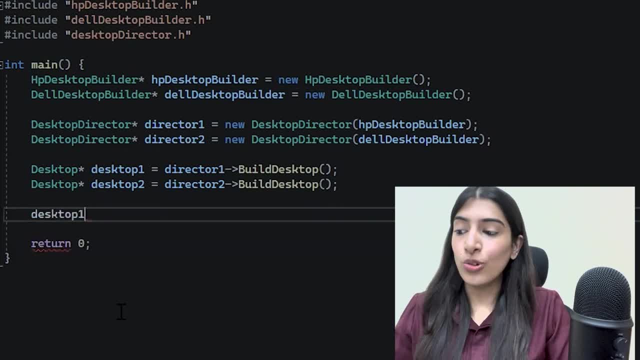 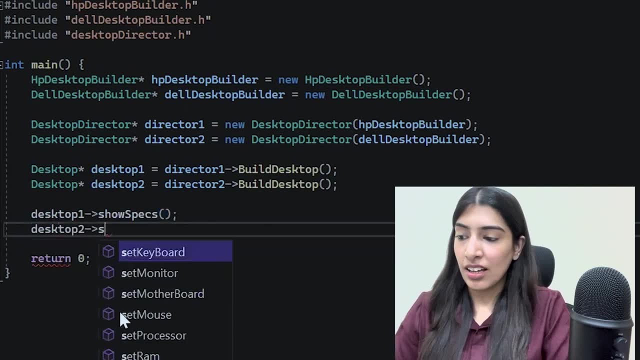 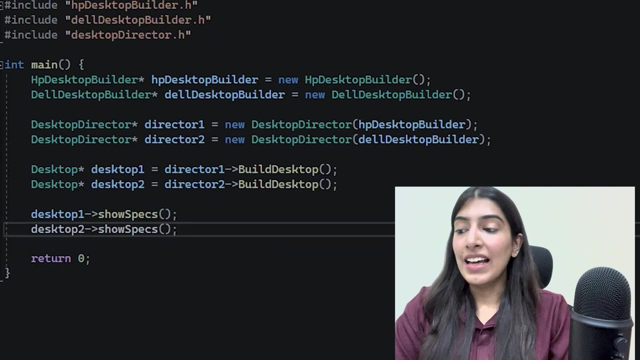 this product right. so to really show you what is being built, i had actually written show specs. remember in the desktop class we had written show specs. so let me just show you that how the uh product has been developed. let's run it and see. i hope everything works. 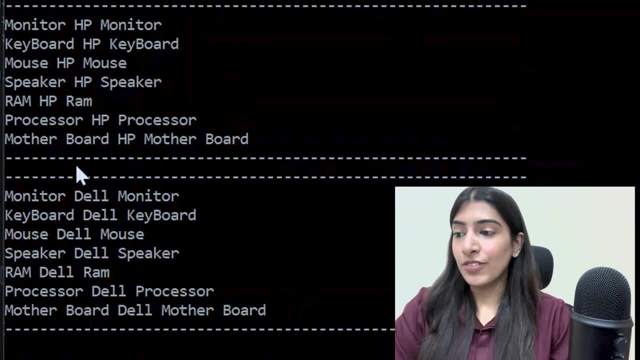 right. as you can see, it looks so beautiful. so first thing that we had passed was hp builder. so first hp monitor, hp keyboard, hp mouse- all of these were built, and then the second desktop, when it was built, or everything was built from there, right? so this is what we have done. 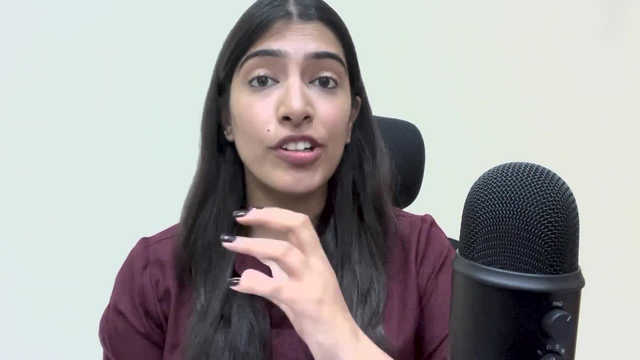 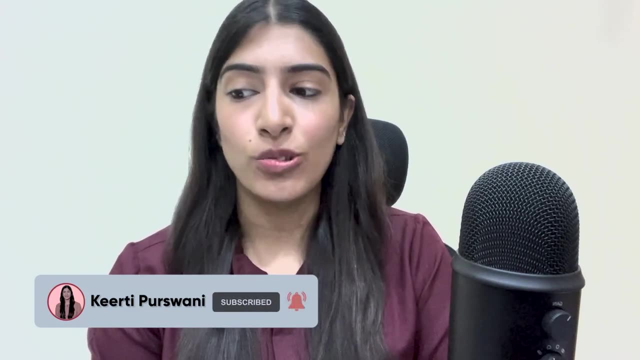 so, as you can see, we've made the entire building- a complex object- very simple for our client. what it had to do. it just had to tell: okay, this will be my builder. and it told the director that you know what? use this builder, build the object and